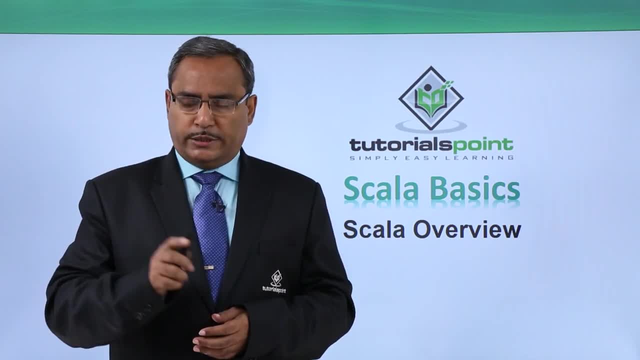 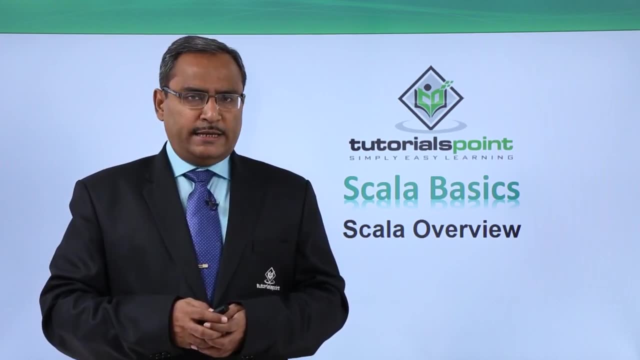 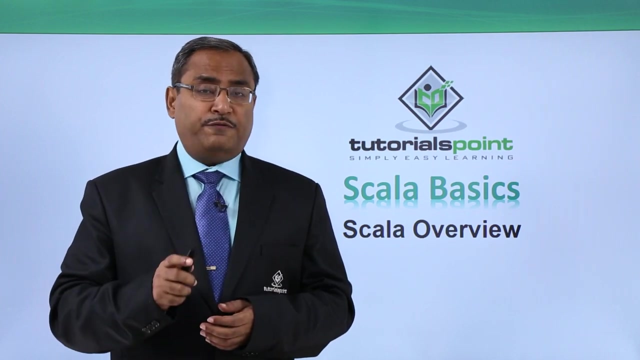 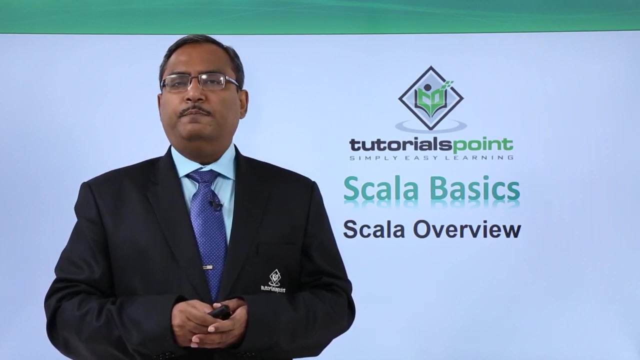 Scala overview. Here in this session we shall discuss different important features and advantages of Scala programming. We know that Scala is a general purpose language. Using this Scala, we can develop multiple different applications, and especially for concurrent applications and distributed applications. As a result of that, in big data, in big data. 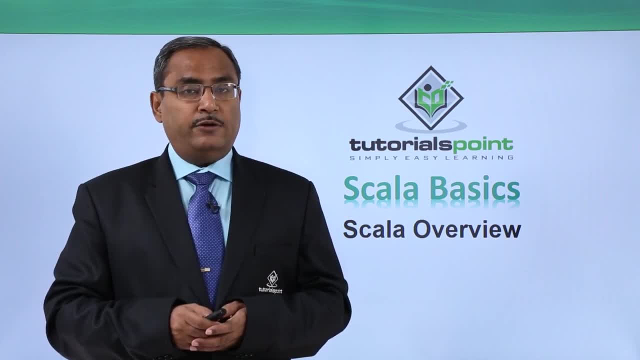 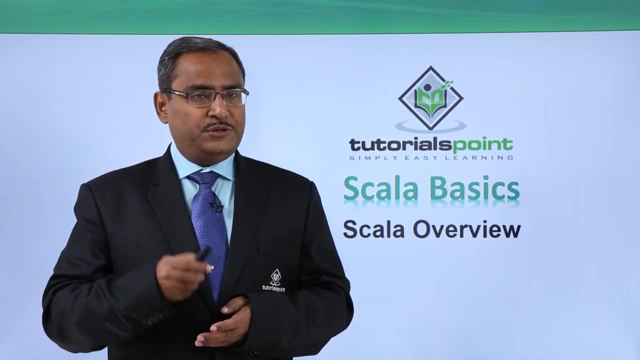 oriented applications, Scala programming is playing a very vital role. James Gosling was the creator of Java. The comment was made by James Gosling was that if he has been asked to select the next language, next programming language other than Java, he would be selecting this Scala. 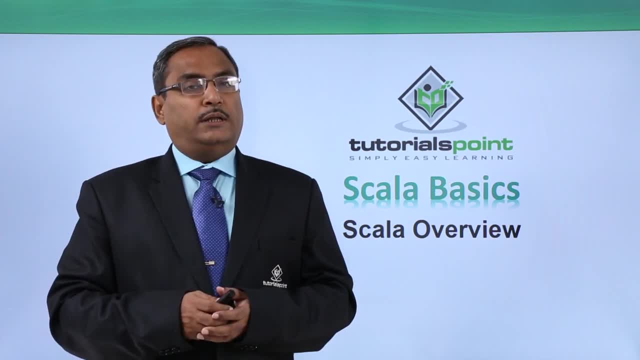 language. So that is very interesting. And also the creator of Groovy, that is James Strachan. he is the creator of Groovy. He is the creator of Groovy. He is the creator of Groovy. He is. 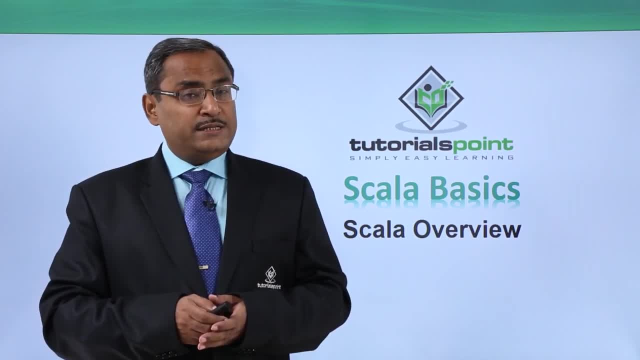 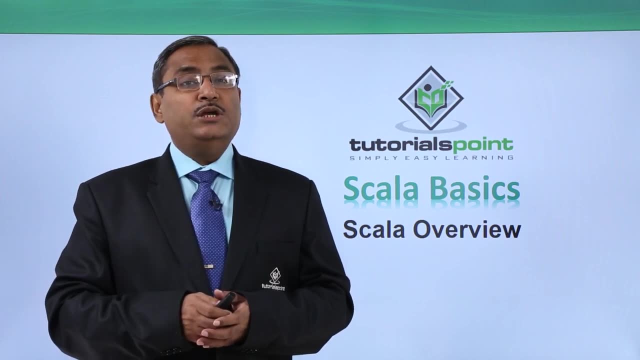 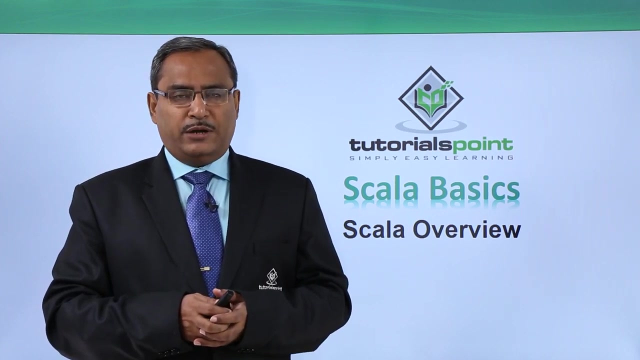 he has made one very interesting comment, that he made this comment that if he would get this programming in Scala book in the year 2003, he would never had gone for the development of Groovy. There is another, another very important comment we got from your Charles Nutter, who was: 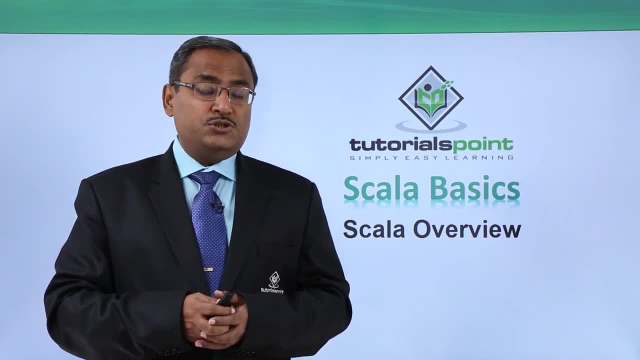 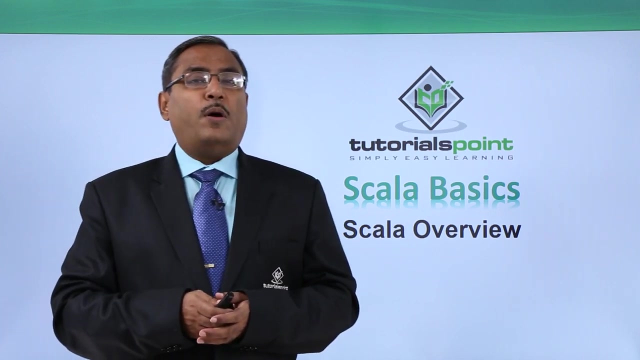 the co-developer of our JRuby. He has told that Java is, Scala is the replacement of Java. So that is why we are getting multiple different comments from different renowned persons regarding this Scala programming. So Scala is getting more and more popular nowadays And, as a trainer, 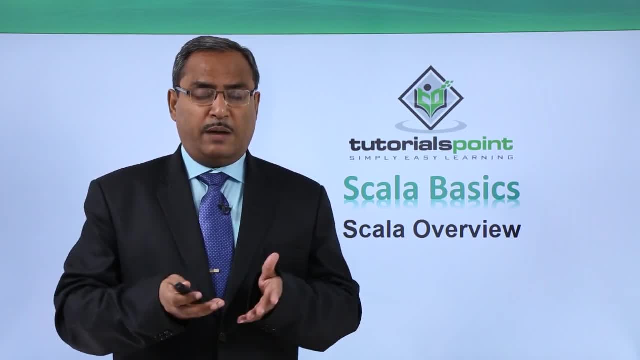 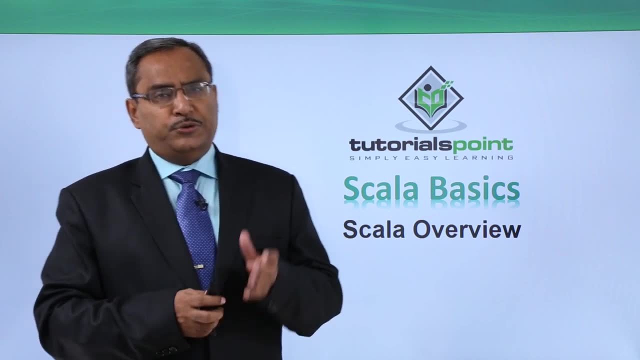 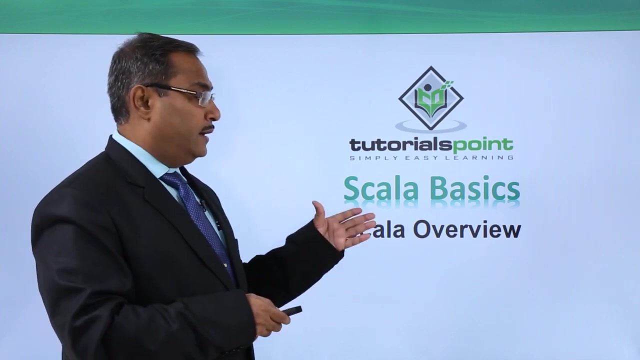 as a developers, from the testers we are getting this, this comment, that this Scala is nothing but updated Java. So that is why this particular tutorial: we will be discussing the overview of Scala, where we will be discussing multiple different points in this, with respect, 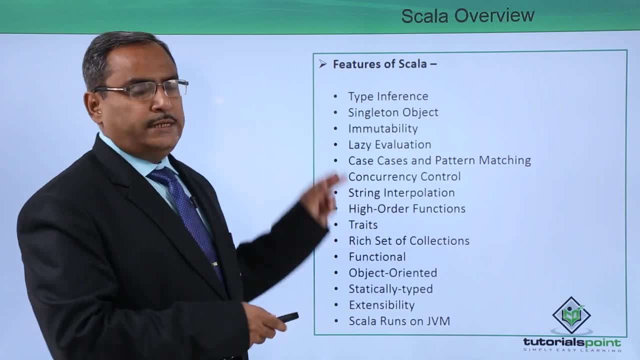 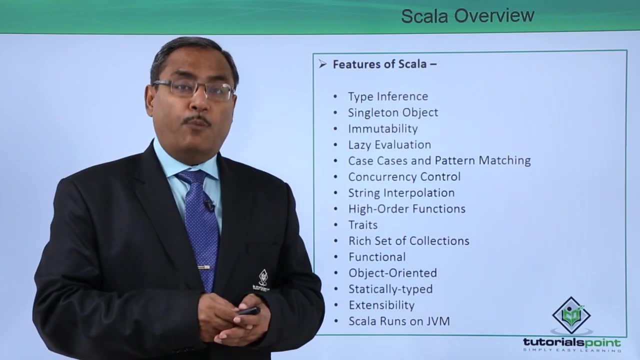 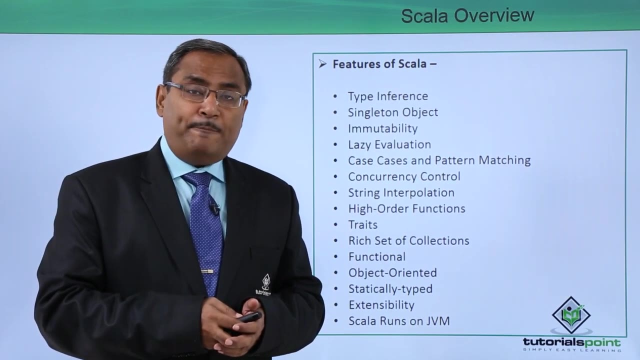 to the topic. So here we have listed some features of Scala. If we go on counting, we have listed only 15 such features, but obviously we can consider more than this list. Scala nowadays, as I have told you that is getting more and more popularity and applicability. 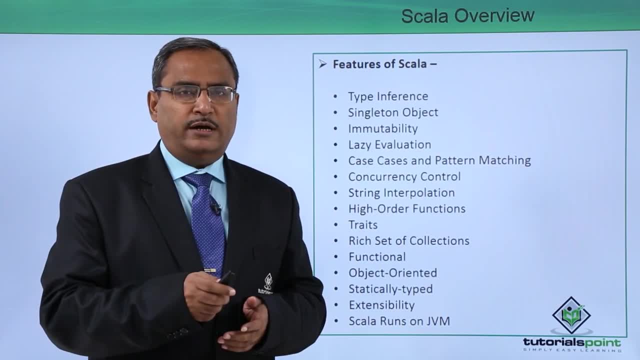 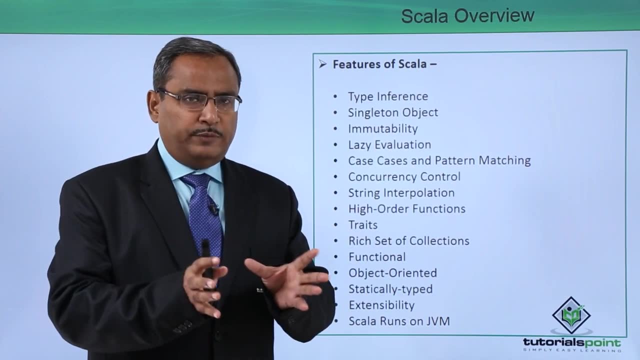 You can consider Twitter, you can consider your LinkedIn, Coursera, Foursquare. So they have transformed. they have transformed and developed most of their major part of their codebase on to the Scala. So that is why Scala is getting more and more popular. So in this, 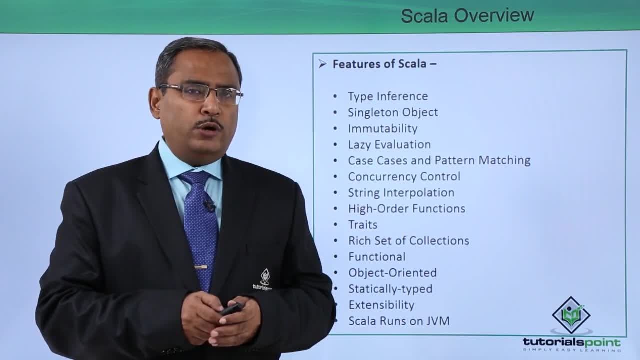 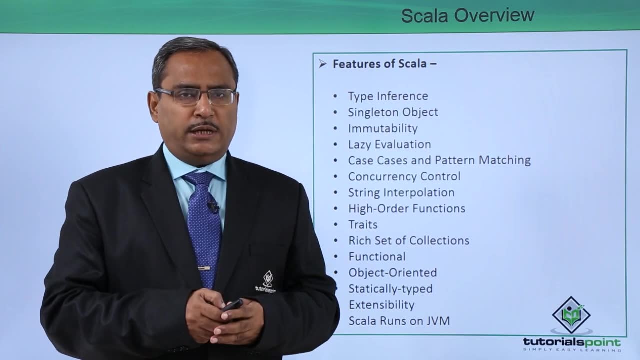 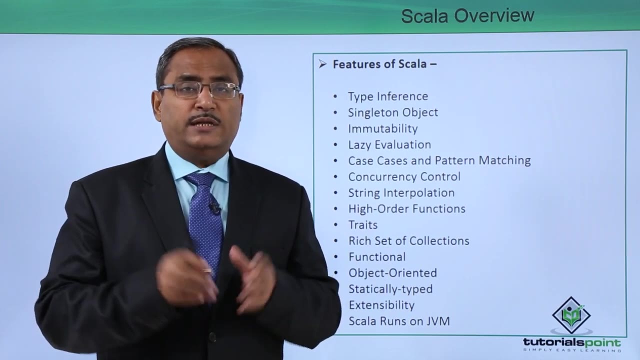 particular tutorial. we will be implementing our Scala code in two different environments: one using the IDE, where we will be writing a complete code and then we shall go for the compilation and then execution. and also we will be using very top level interface, that is, the shell. the shell interface that is known as REPL, that is a read eval print. 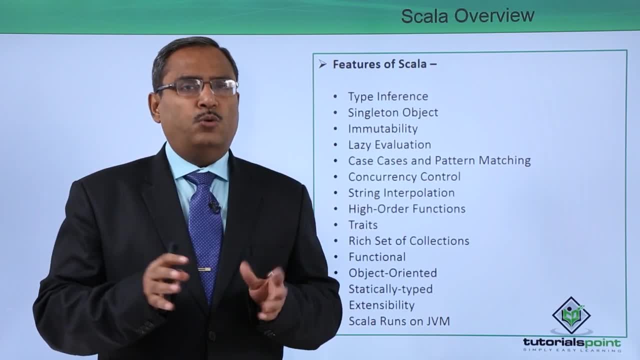 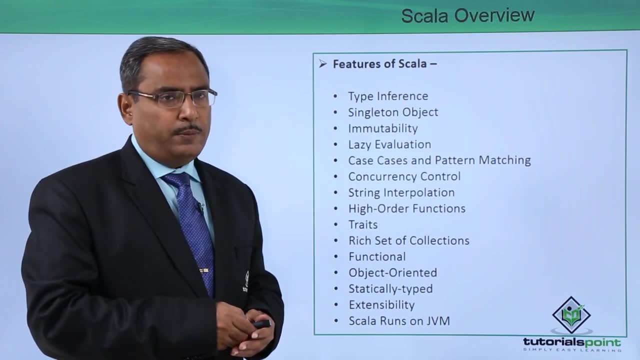 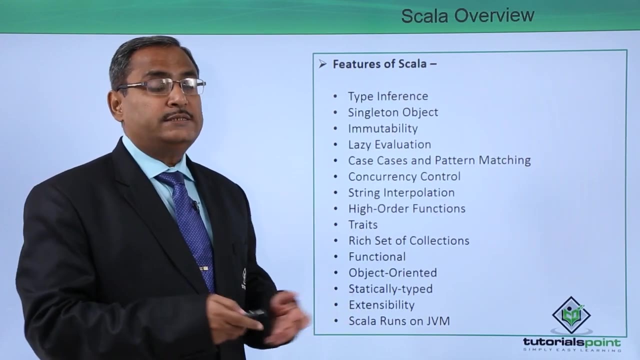 loop. So there also, in a very interactive way, we can execute line by line in the shell environment. So let me discuss all these features one by one. So the first feature we are considering, that is a type inference. Now question is coming in mind: what is type? 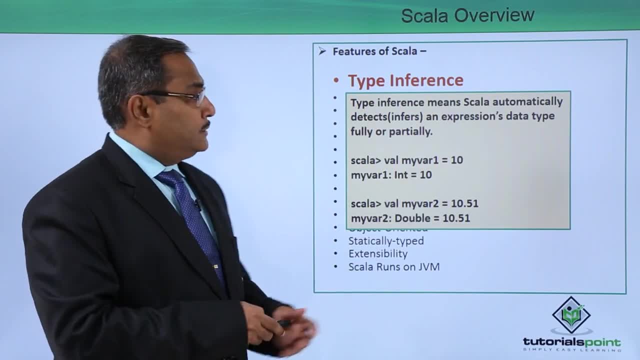 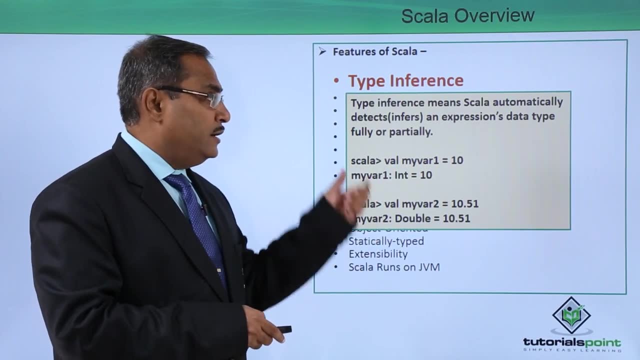 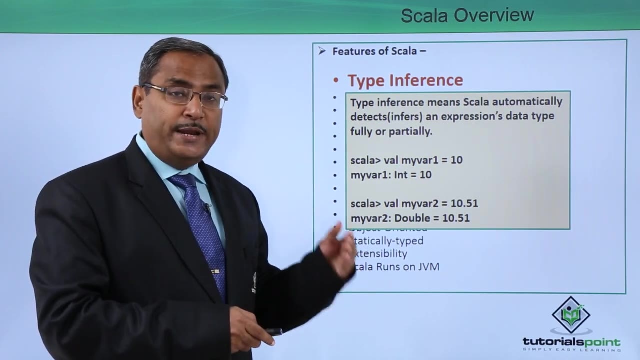 inference. So this is our type inference. So type inference means Scala automatically detects or infers an expression's data type fully In the REPL environment, that is our read eval print loop environment, that is, in the shell environment- we have written this particular assignment statement. that is a. 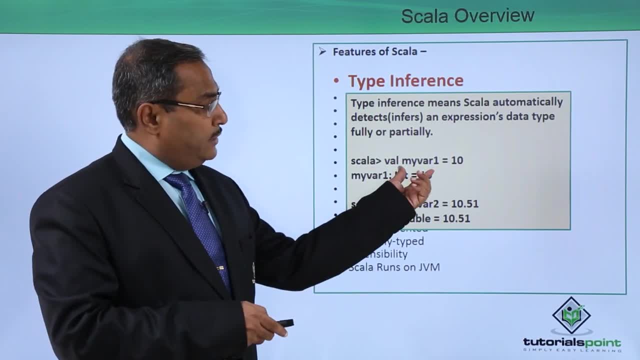 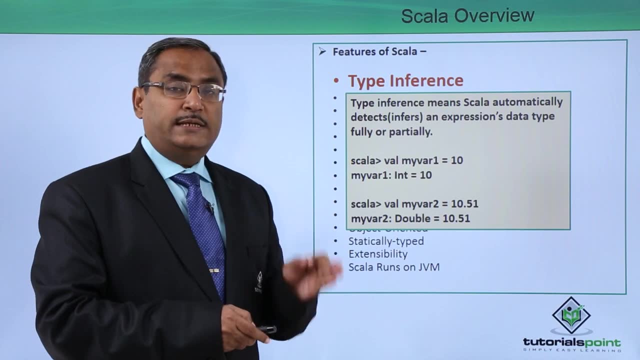 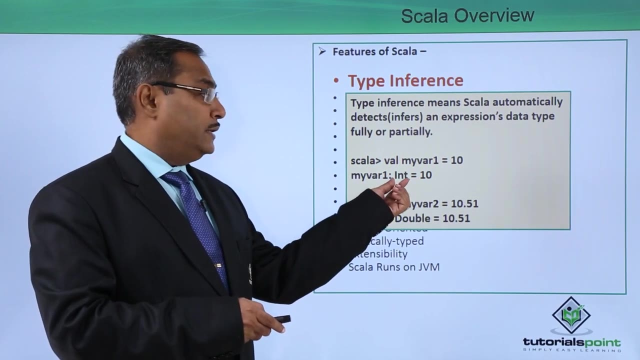 val, my var 1 is equal to 10.. Here you see, we did not mention the data type of my var 1 explicitly, but due to the presence of the feature, there is a type inference in Scala. So now it has been interpreted as it is of the type. it is of the type. 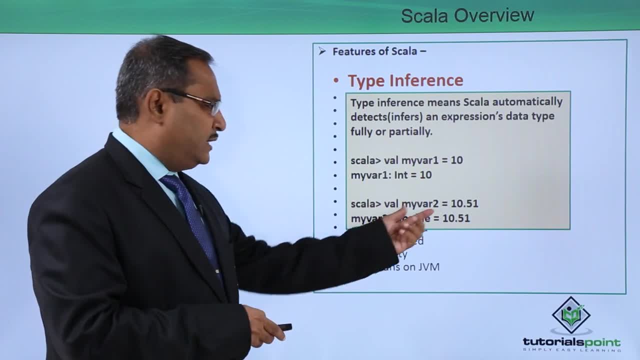 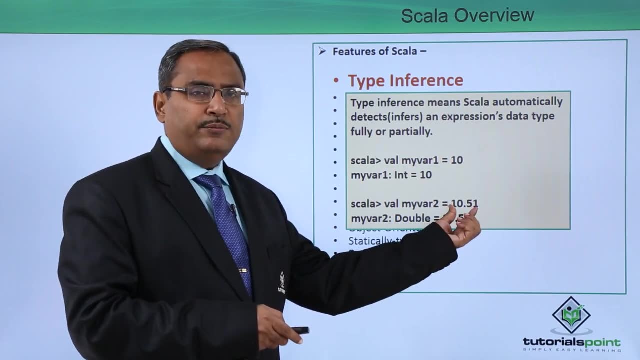 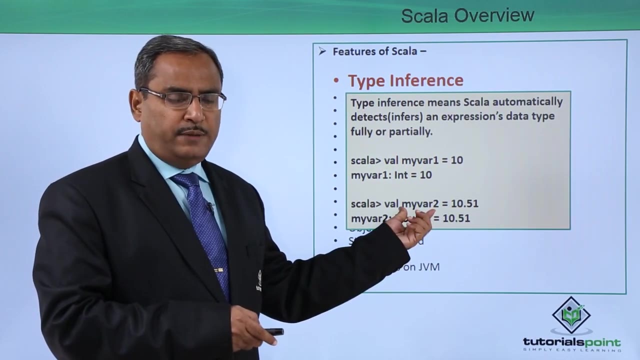 int and getting the value 10 here, Just change the respective initialization value. So here we have written val. there is a. my var 2 is equal to 10.51.. So whenever I am assigning 10.51, irrespective of the fact that I have not mentioned the data type for my var 1,, 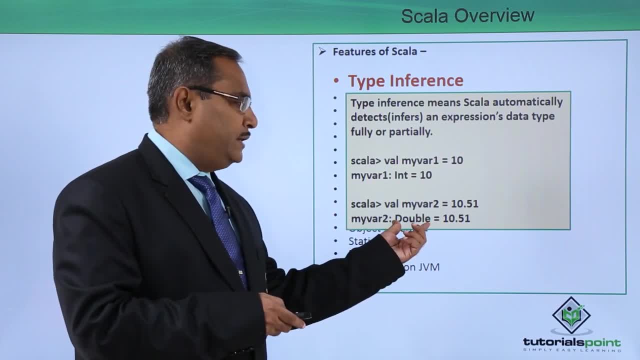 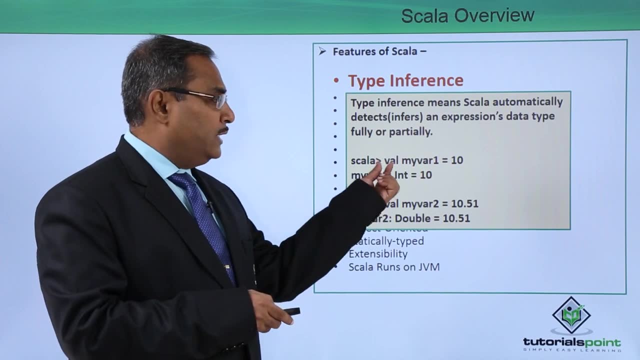 so my var 1 is getting inferred as of the type double and has got initialized with the value 10.51.. So this property is known as type inference. We know that in case of val, whenever we are defining one variable, in case of val, whenever writing. 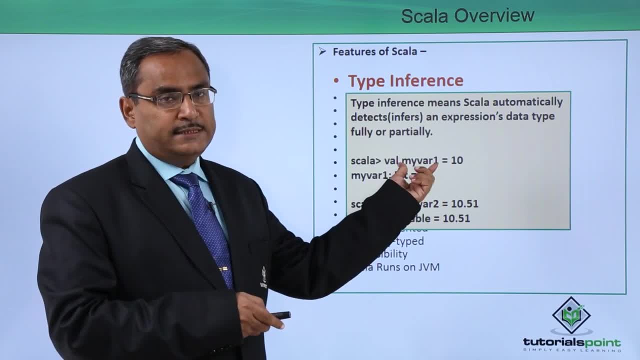 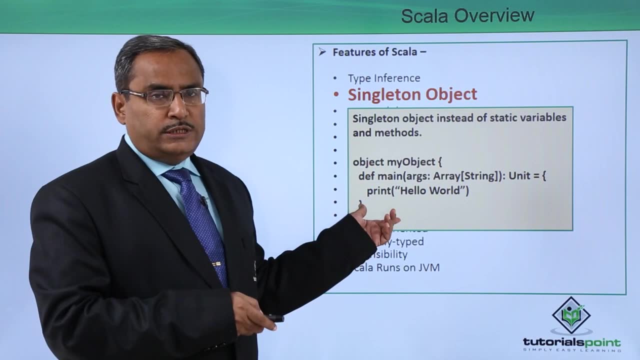 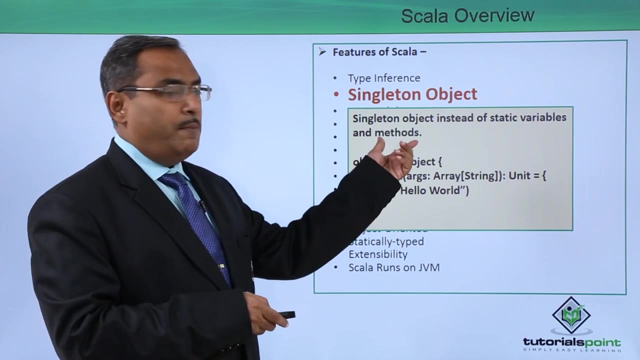 val my var 1,. that means it is getting defined as immutable variable. that means the value of the variable cannot be changed. Now the next property we are going to discuss is known as singleton object. So singleton object instead of static variables and methods. 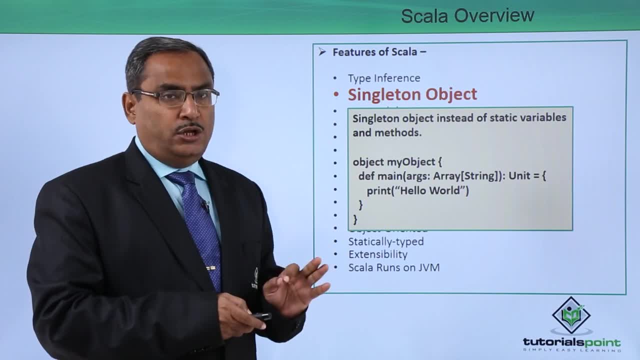 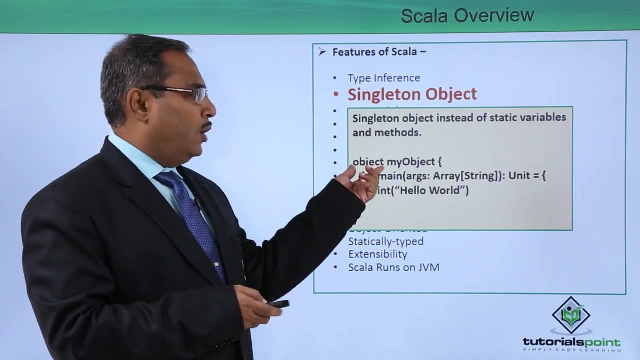 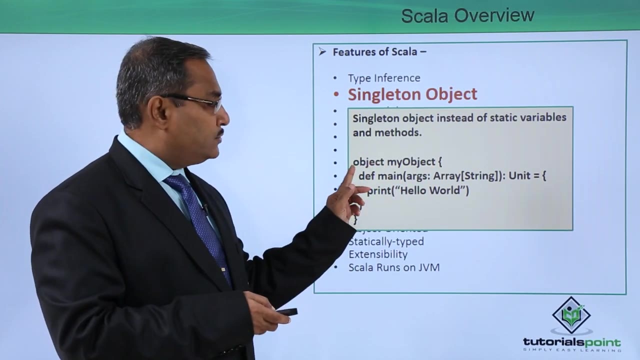 In our Scala there is no keyword called static. So using this singleton object we can, we can simulate the environment of static, That is, let us consider object my object. So here we have defined one singleton object with this keyword: object. Just remember this. 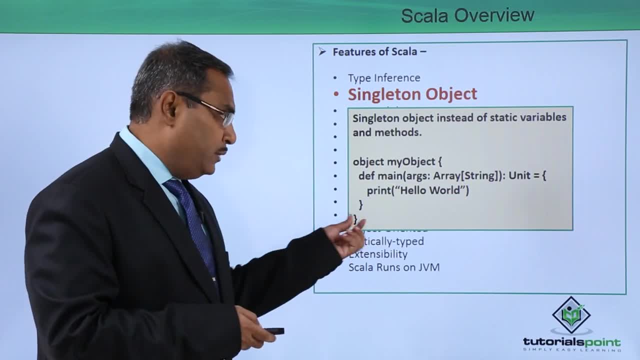 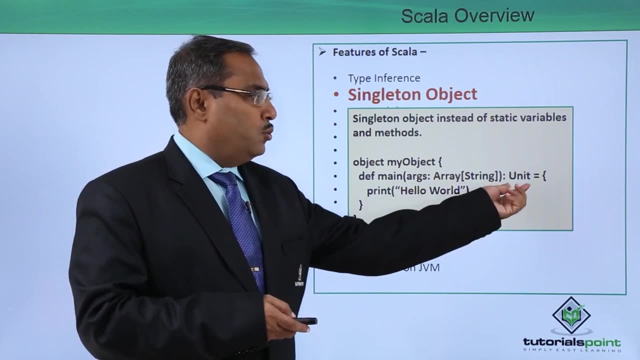 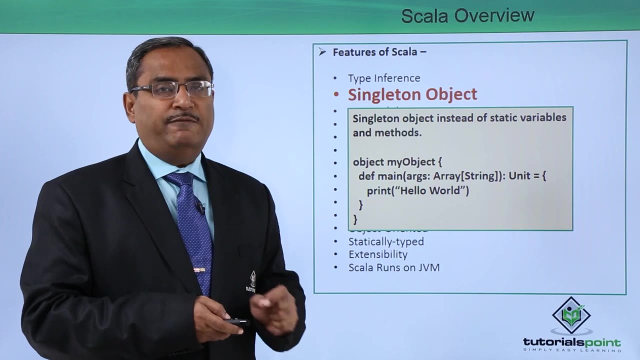 object is having, all the letters are in the lower case. So here we have defined one function. that is our def main. args, colon, array, strings. colon unit is equal to. this is the respective code here. So this very line is defining our main function. 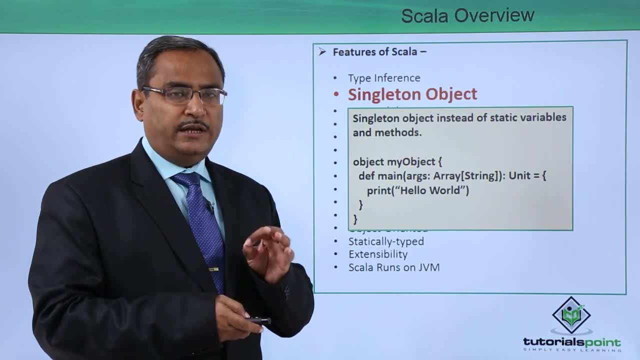 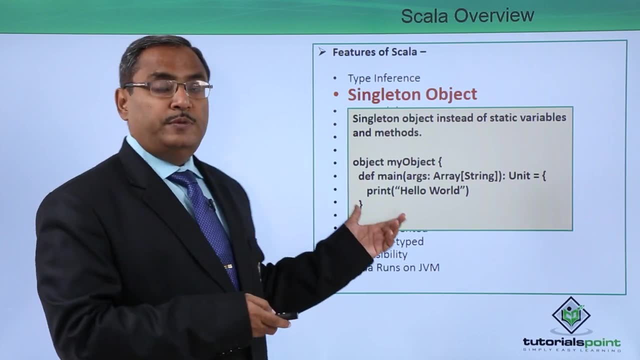 In our, in our Java programming we used to write the main function having the default prototype like like public static void, main string, arg. So here also we have. we are going to write the same, but in the Scala syntax, So as a static keyword is not there present. 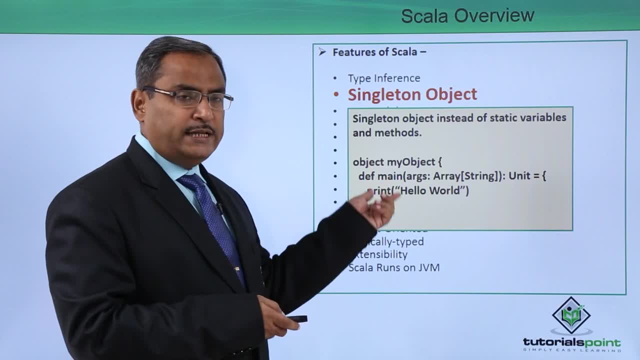 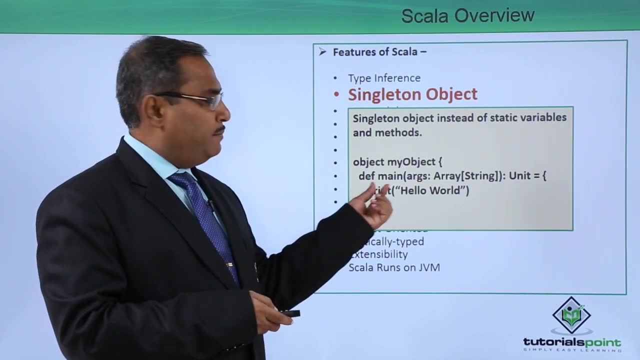 in Scala. so that is why we have written this. we have defined this main function under this object, my object, And this my object is a singleton object. So def means define, main is the name of the function It is having the 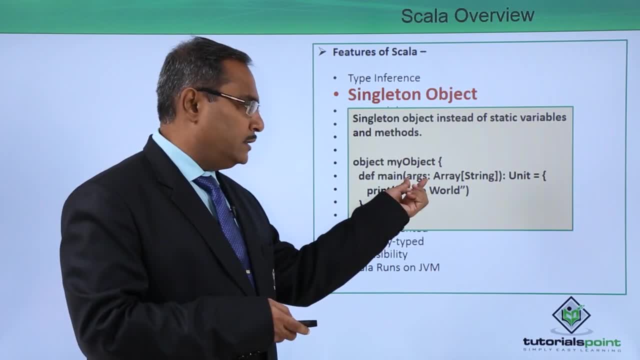 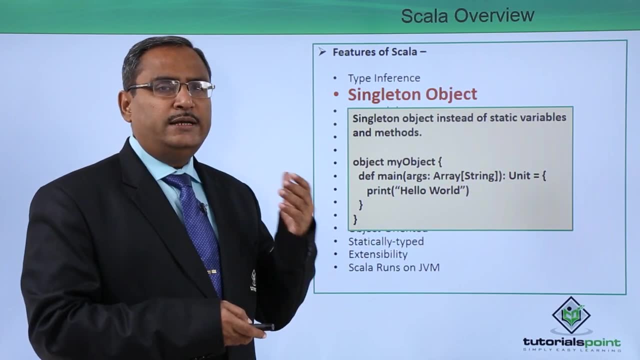 args. there is a argument name. that is the argument name. we are having this- args, which is of the type array, of type string, and which returns void. So here, unit denotes and nothing. that is the void here and which is equal to which is having this respective body there. 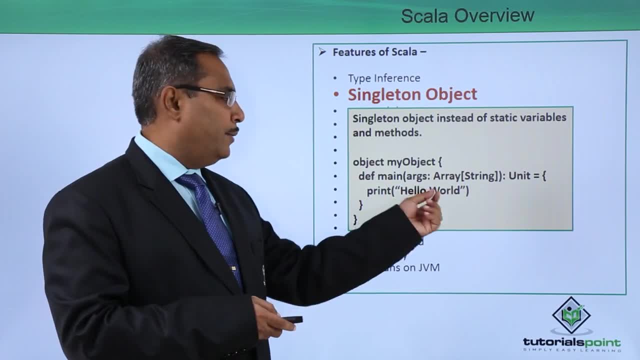 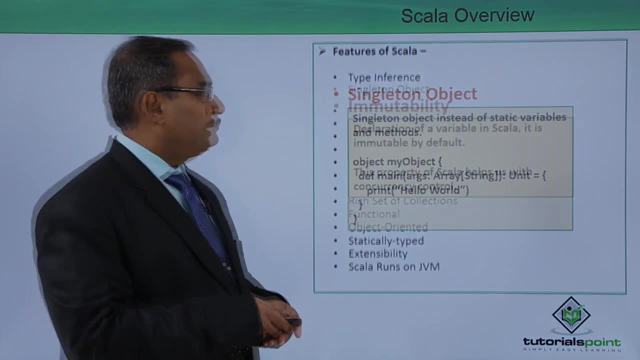 is a print, hello world. So hello world is a string, must be enclosed within double quotes. So this is our singleton object. So that is one of the features of this Scala programming. The next feature we are going to discuss is known as immutability. So declaration of 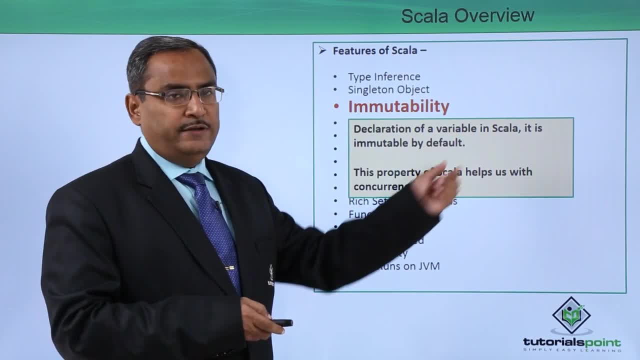 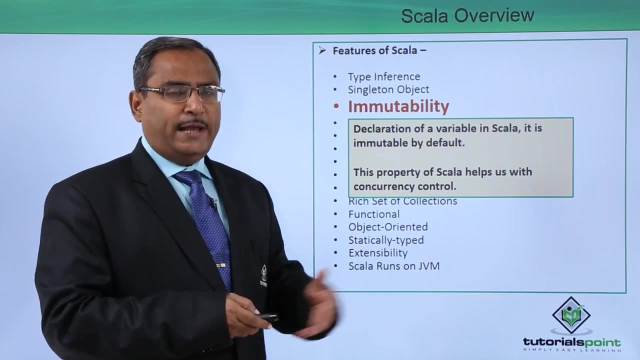 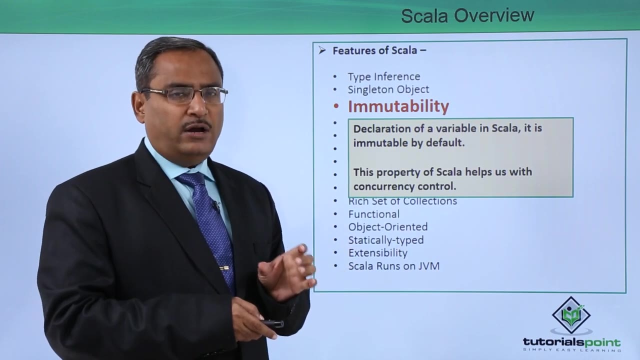 a variable in Scala, it is immutable by default. So this property of Scala helps us with the concurrency control and also to develop applications in the distributed environment Whenever we define one variable, that is, let us suppose we are writing this- val my var. 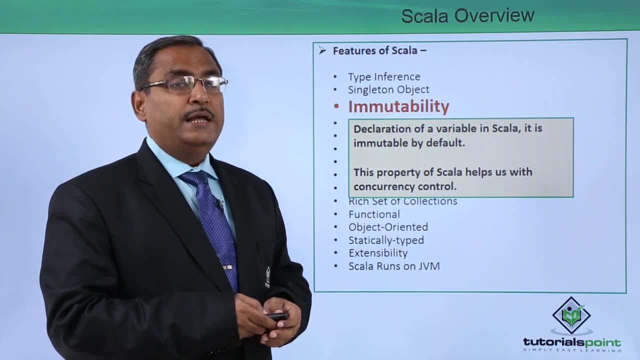 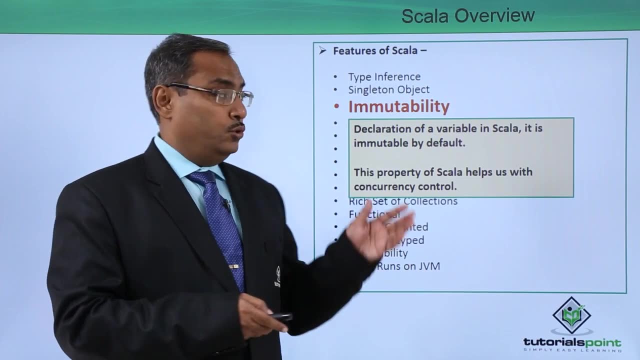 1 is equal to 10, this, my var 1, is becoming one immutable variable. So this, my var 1, is a variable. that means the value of this, my var 1, cannot be changed, cannot be altered. So this particular property, there is a immutability. this property of Scala helps us to develop. 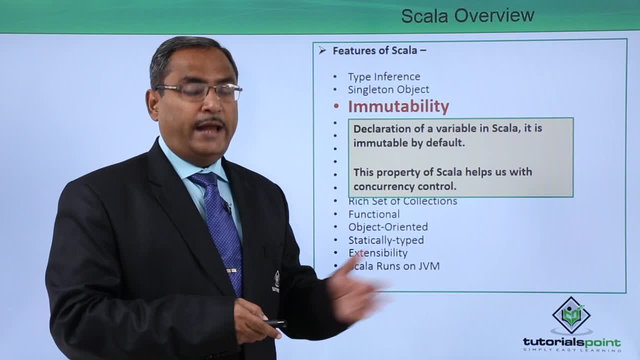 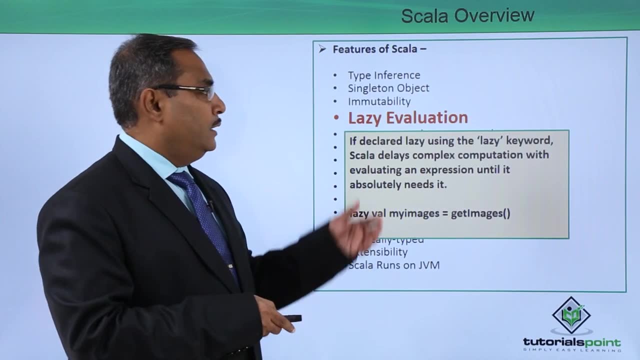 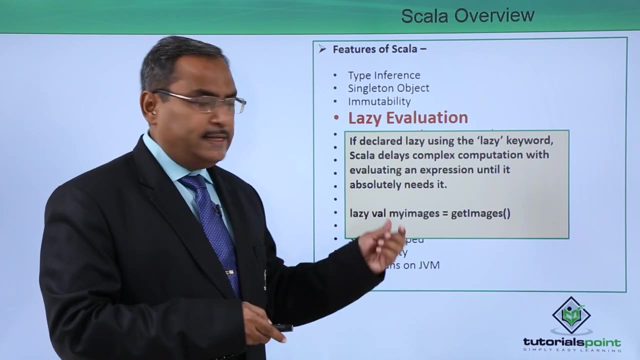 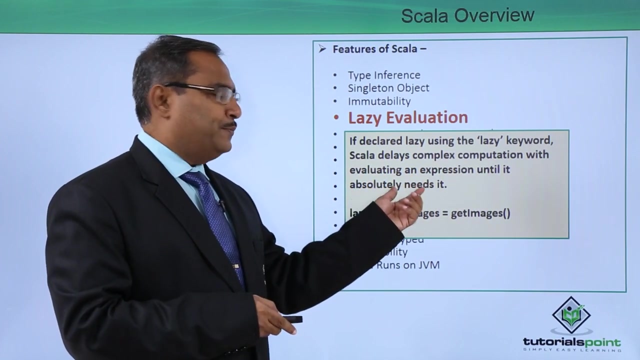 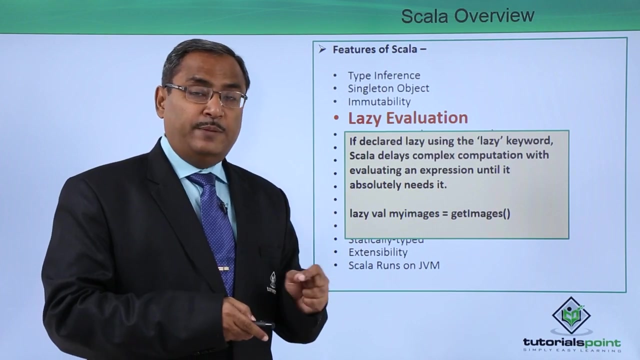 applications which are capable to handle concurrency and also capable to work in the distributed environment. Next one: the property is known as lazy evaluation. If declared lazy using the lazy keyword, Scala delays complex computation with evaluating an expression until it is absolutely needed. So that means whenever we are defining one variable with the lazy keyword, then the variable. 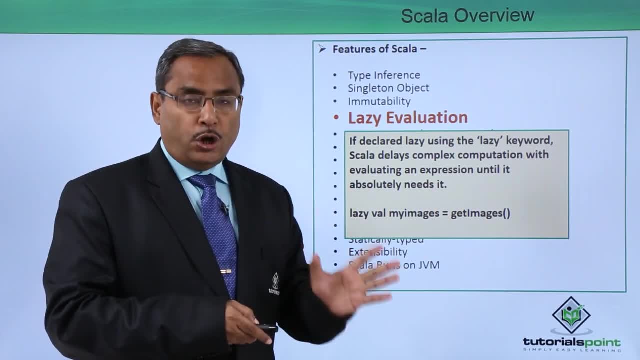 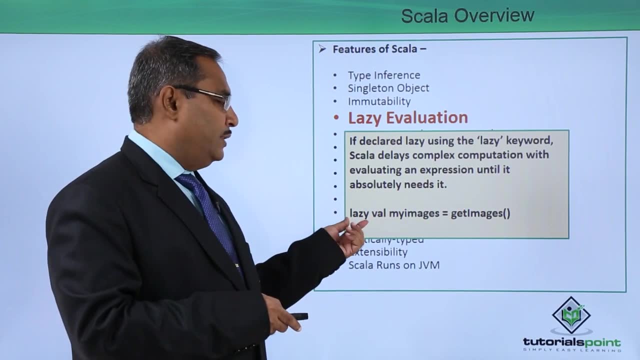 that will be evaluated whenever it is declared, not prior to that. So only on the demand the variable will be evaluated. So just consider this example here. So lazy val my images is equal to get images method. So here you can find that this particular my images is. 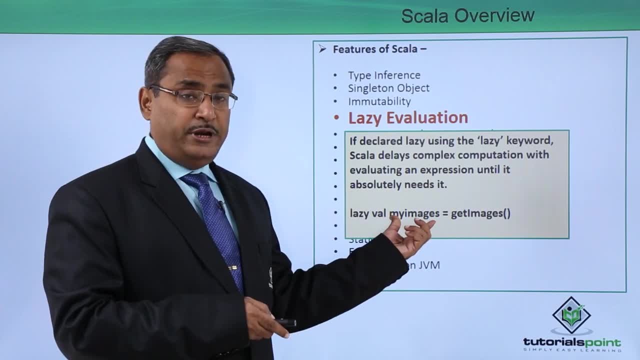 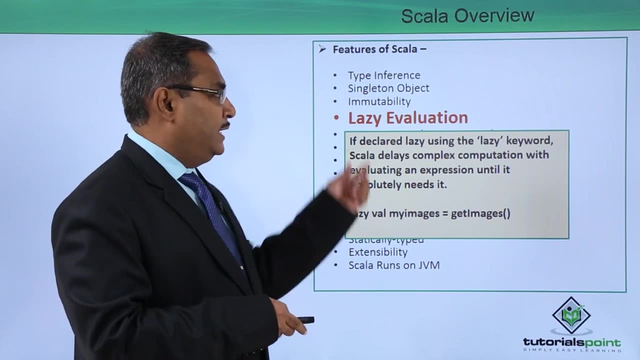 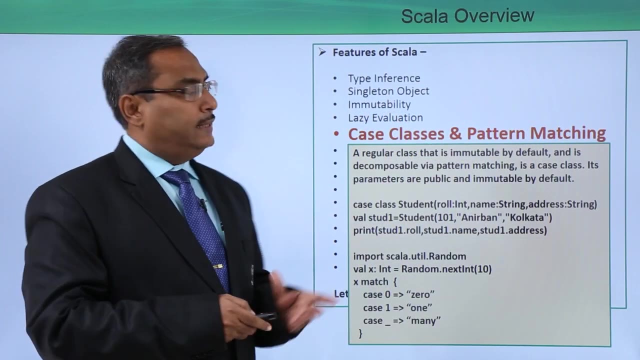 this particular variable will be evaluated as when required, not in prior, because we are having the preceded this keyword, that is lazy. So that is why lazy evaluation is one of the features of Scala programming. So the next property we are discussing, that is our case, classes and pattern matching. 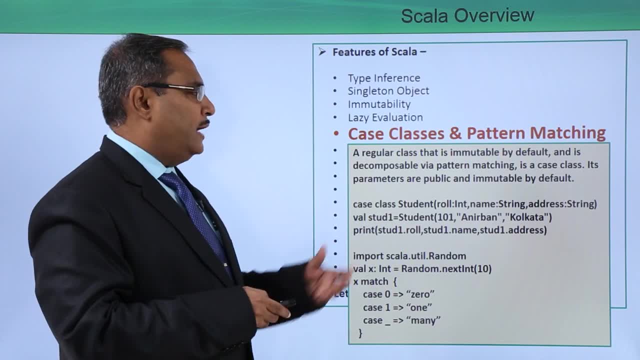 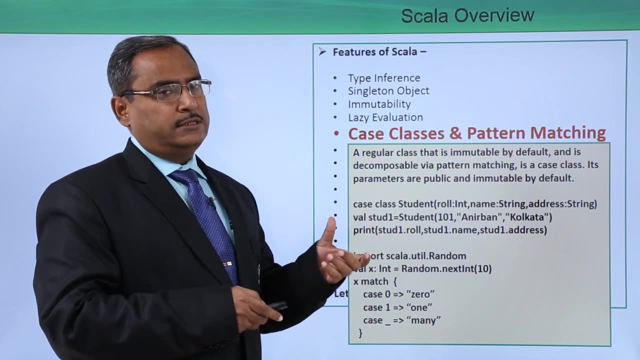 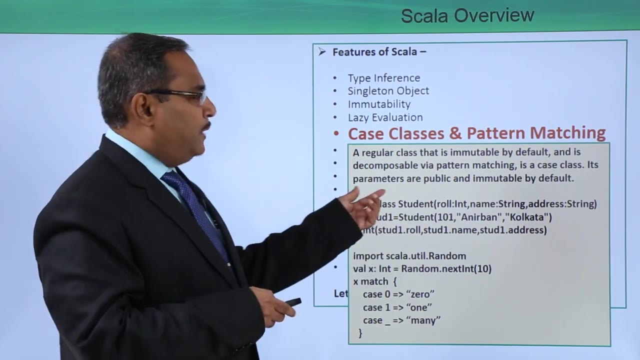 So a regular class that is immutable by default and is decomposable via pattern matching is a case class, And while writing a case class, the case class must be preceded with this respective keyword. that is a case and class, And its parameters are public and immutable by default. 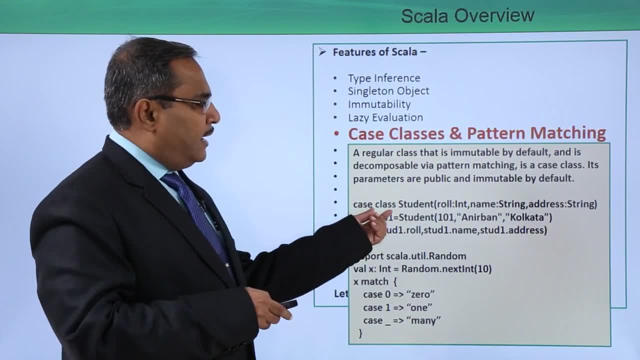 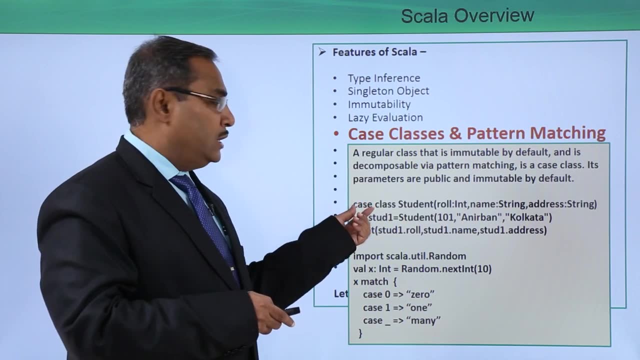 So let us go for one example to show you that case class student. So here you see, we have written this case class. While writing this case class, we are supposed to mention these keywords. So case class student. So there is a respective class name. It is having 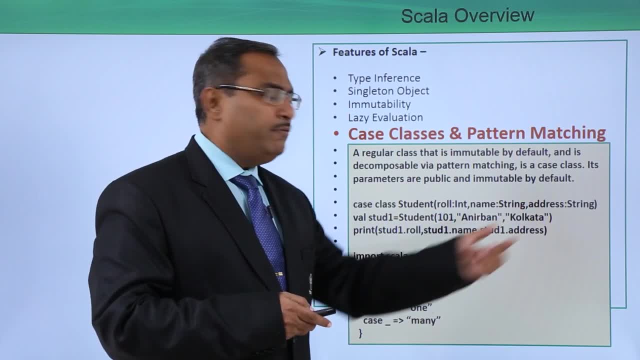 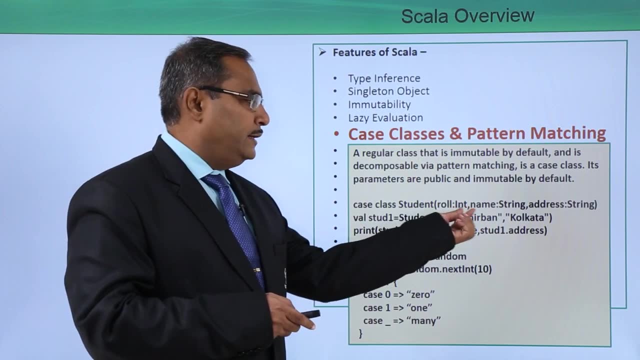 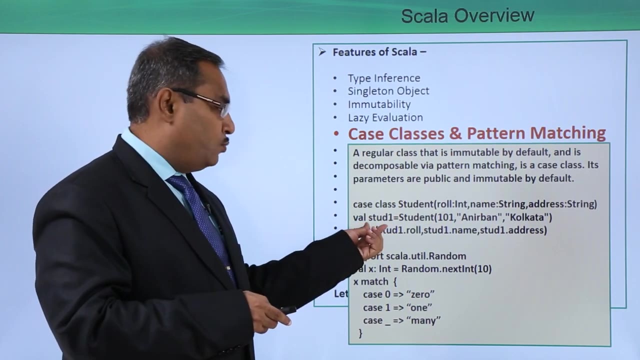 say role of the type int name. So I have very few arguments here, So I will tend to be more transparent here. there is role of the type int name of the type string and address of the type string. So three arguments are there. three respective parameters are there. 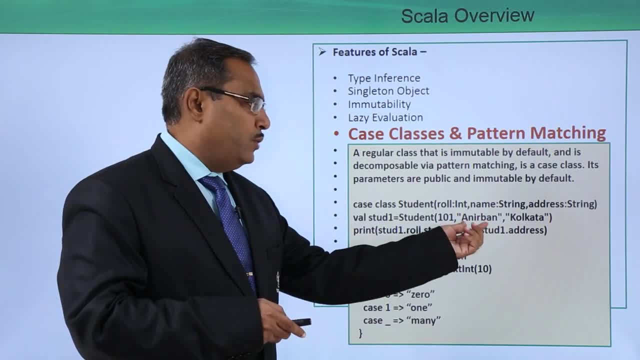 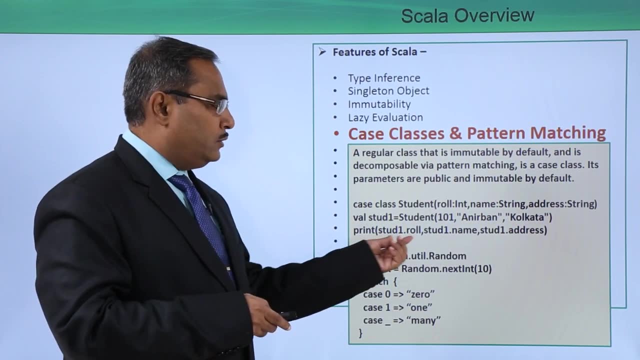 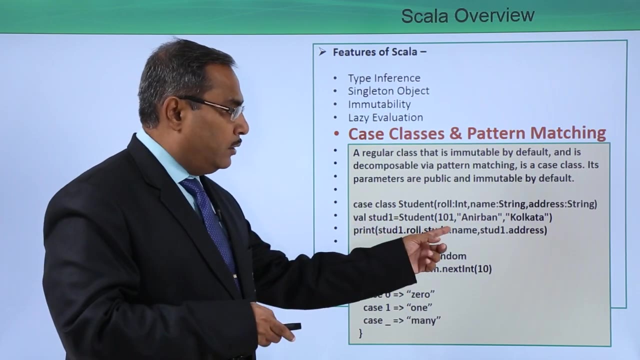 So role of the type int, name of the type string and address of the type string. So now we are defining val, student 1 is equal to student And for at for his role, we are passing 101.. student 1 dot name, comma. student 1 dot address. then it will print 101 anirban and kolkata. 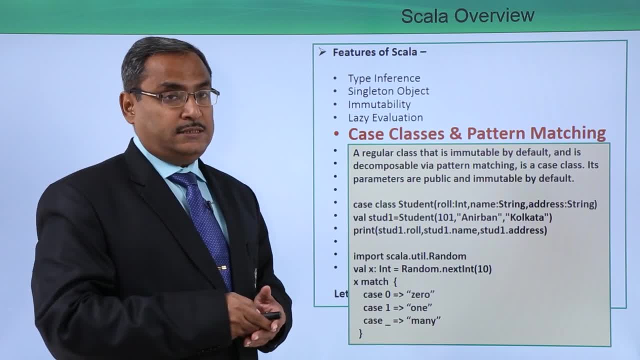 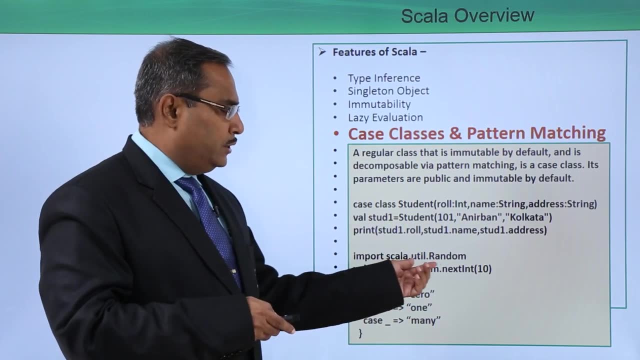 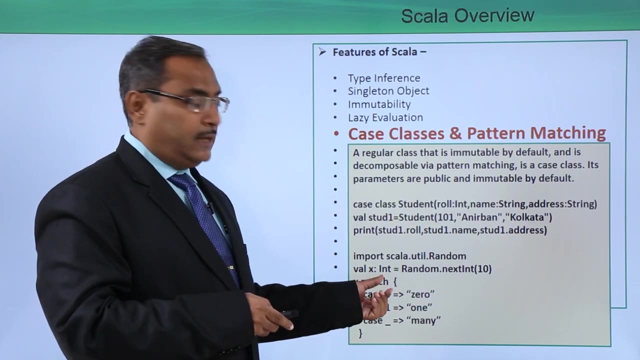 respectively. so there is a utility of this case class in our scala programming now in case of pattern matching. so here we are having this import scala util dot random, because we will be using this random, the respective class we will be using here. so well, x, which is of the type int, is equal. 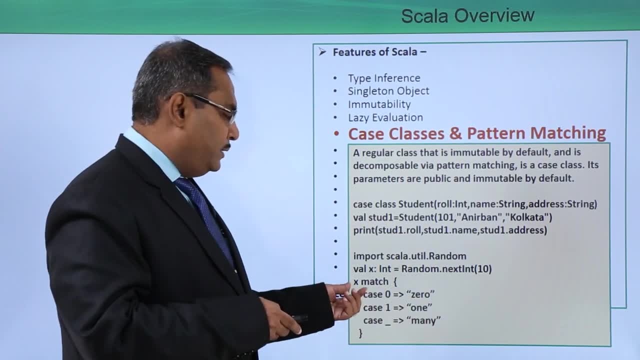 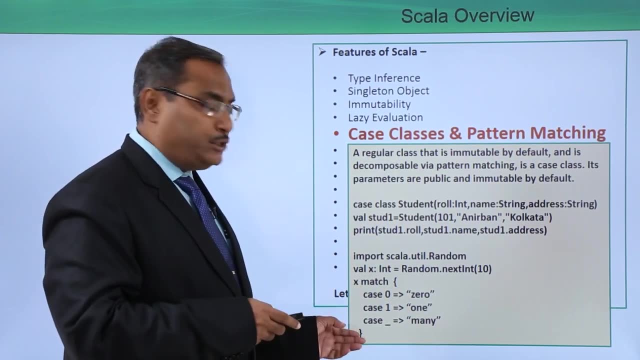 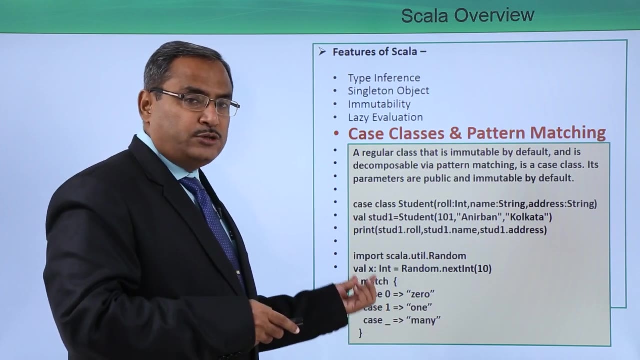 to random dot, next int, and the range is 10. so now x match. so now we can see replacing multiple, if else statements. we can use this respective match here. so case 0: when this x will have the value 0, then the respective 0 will be there. when the case 1, when the x will have the value 1, then 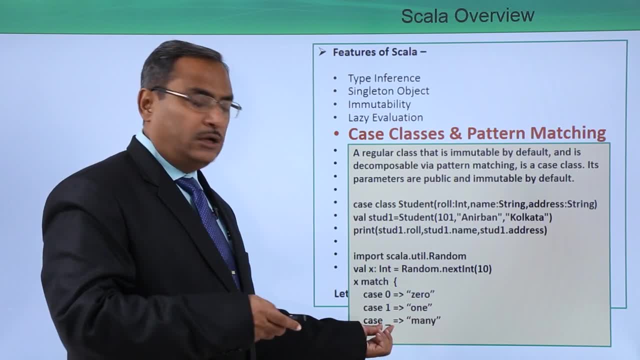 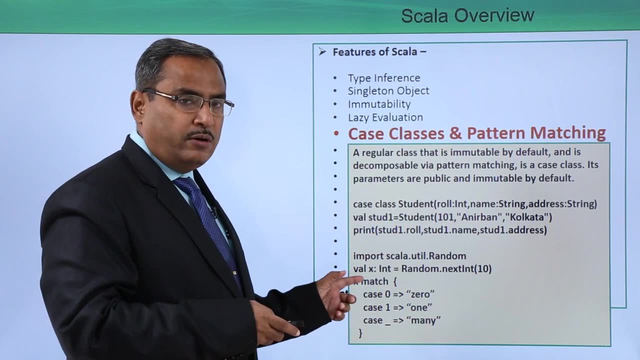 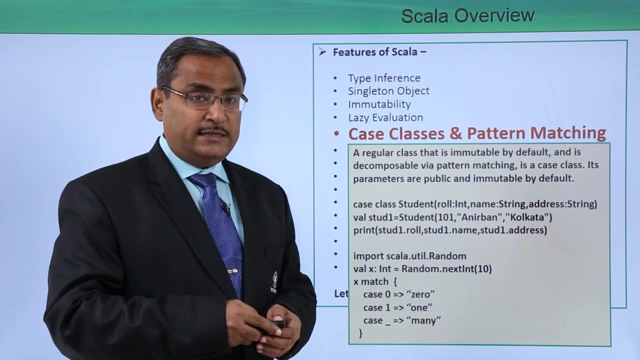 1 otherwise. so here we have mentioned underscore, otherwise will be will be having the string many. so in this way we are doing this pattern matching. depending upon the value of x, the respective string will be selected. so this is one of the features of scala. that is the case. 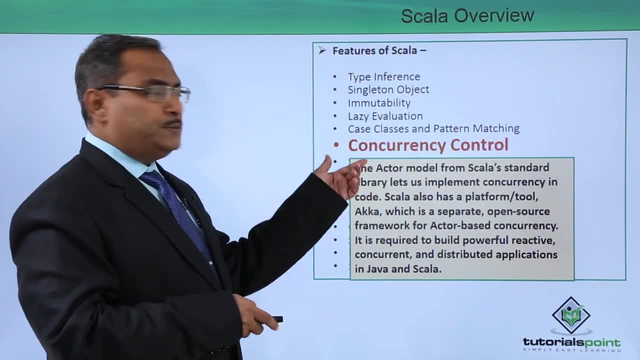 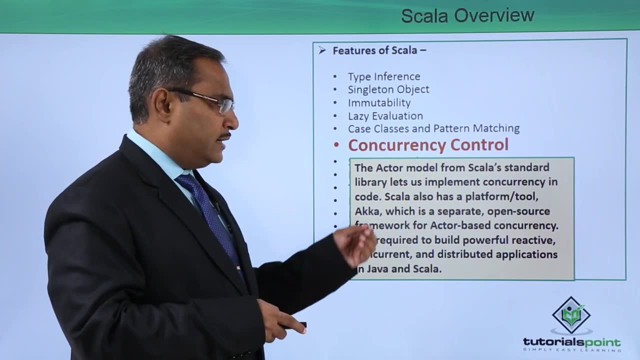 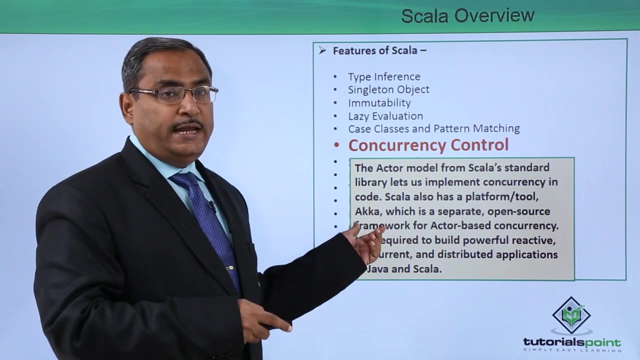 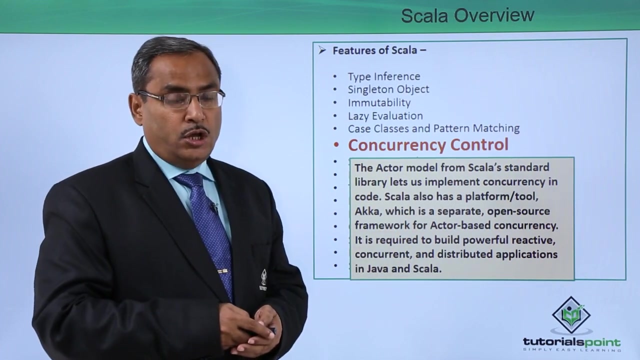 classes and pattern matching. next one, next property is known as concurrency control. so the actor model from scala's standard library lets us implement concurrency in the code, and scala also has a platform or tool, that is akka, which is a separate open source framework for actor based concurrency. so in case of concurrency or in case of concurrent programming, scala is very 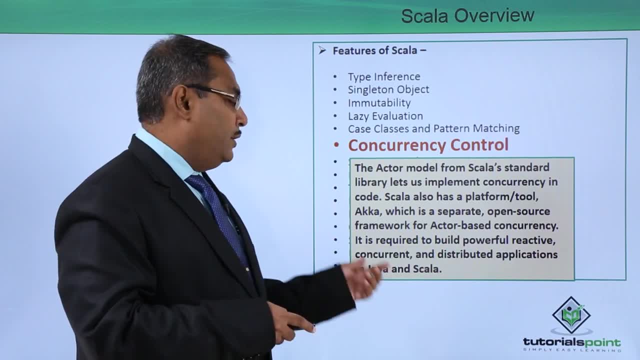 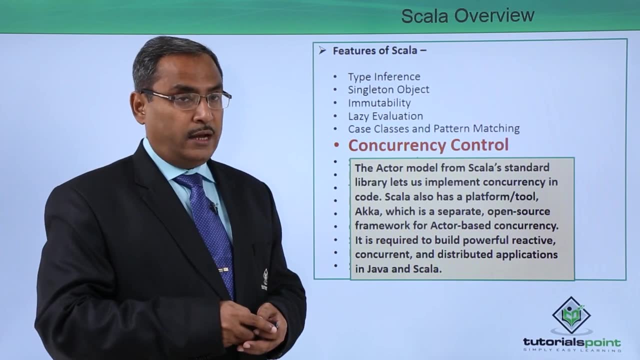 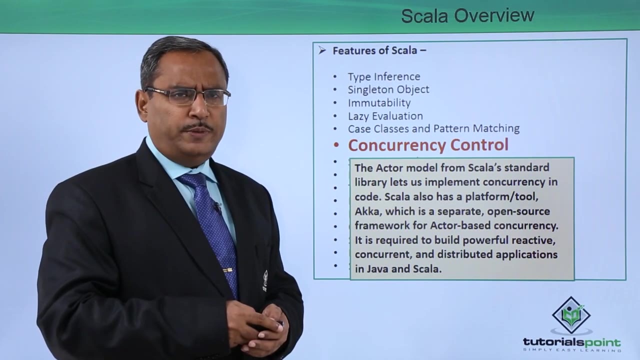 much suitable and it is required to build powerful, reactive, concurrent and distributed applications in java and also in scala. so that feature is known as that is a concurrency control. so in case of distributed environments, multiple transactions will be there, multiple threads will get executed. so concurrency control is very much required in the code. so that's how we are able to implement. 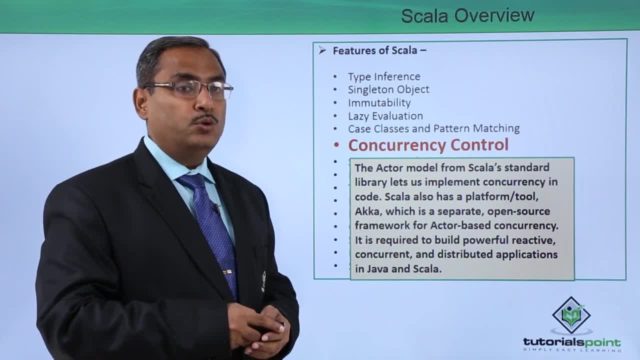 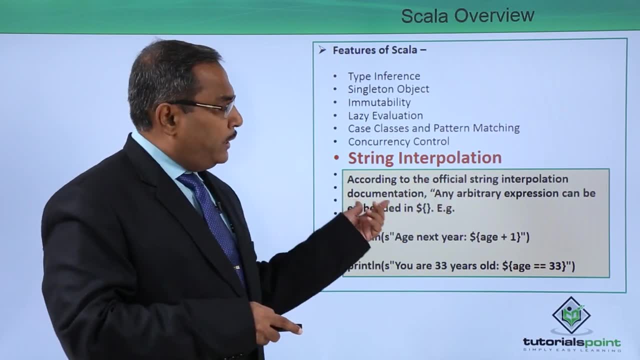 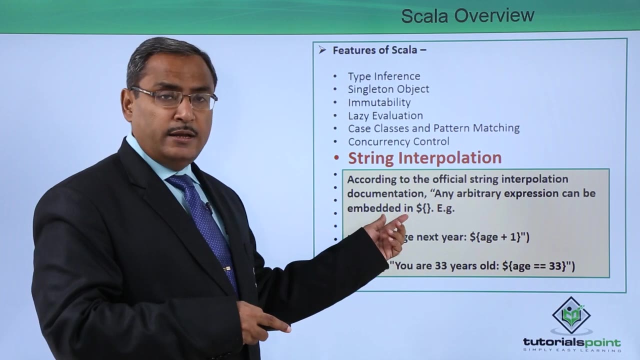 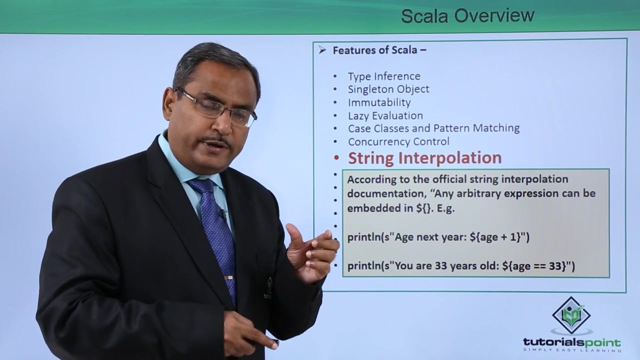 in those applications and scala is very much suitable for those applications development. we are having the string interpolation, so according to the official string interpolation documentation, any arbitrary expression can be embedded in dollar, then within curly braces. so here we can put any kind of expression. the expression will be evaluated and the value will. 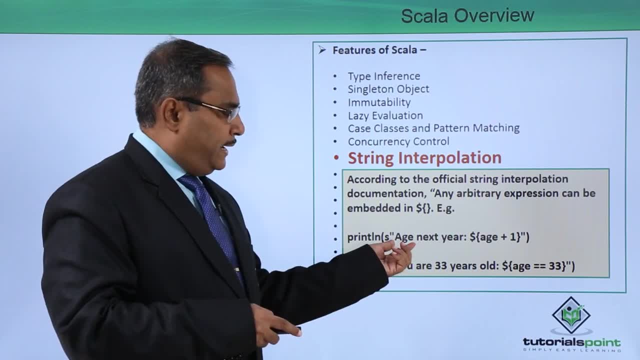 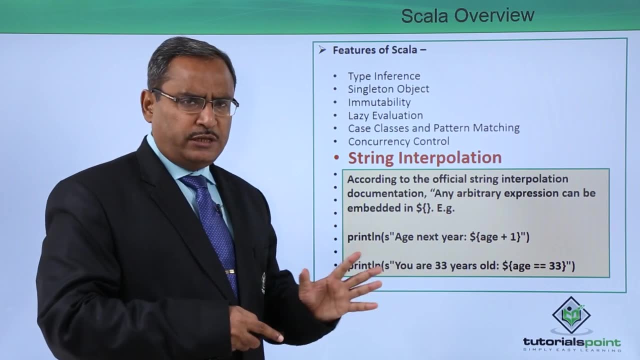 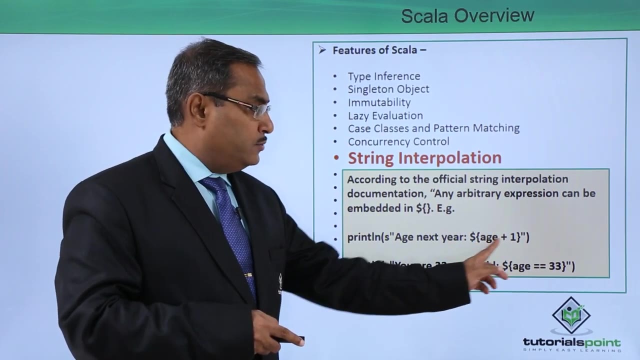 be obtained. so as example consider this one. so age next year is equal to h plus one. here you see we are having one expression here. let us suppose initially the value of age is 40, so 40 plus 1, that is 41. so here we are having this dollar, and then within curly braces we have 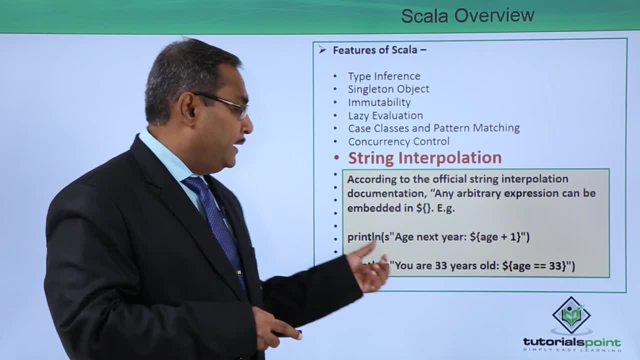 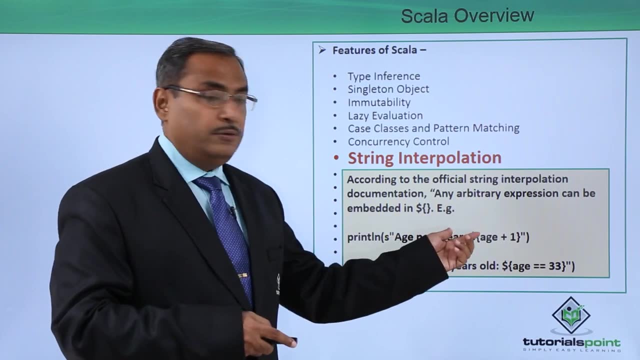 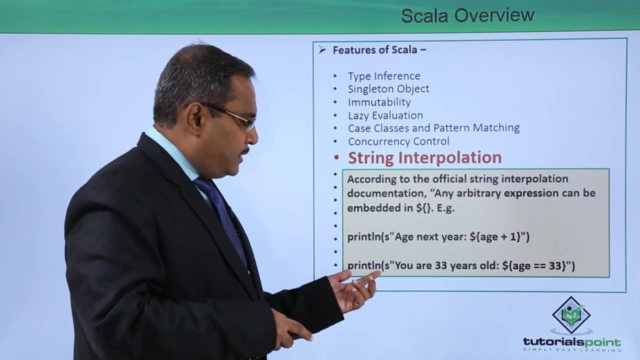 written the respective expression. so that is 40 plus 1 here, and it will be treated as a string. it will be treated as a string. so now, in this way, the age next year is equal to 41 will get printed when this particular code will be having its execution. so just consider this so. 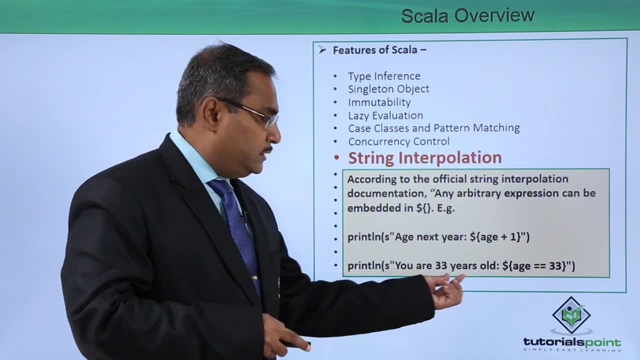 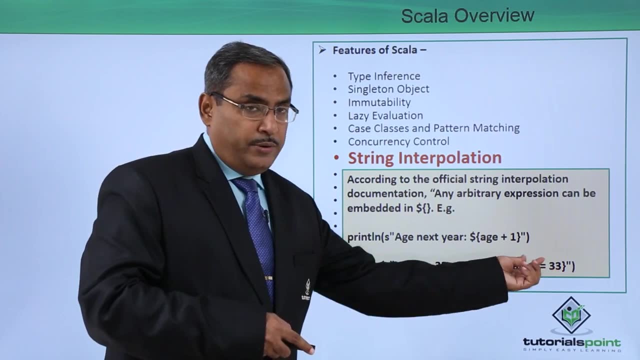 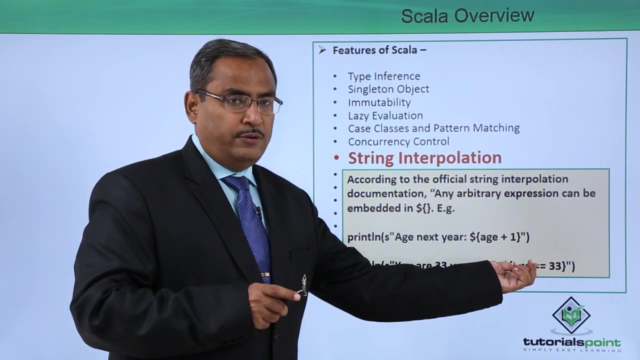 println s, that means the string. so you are 33 years old. so in that case you see, this age double equal to 33. so now here we are, checking whether this age is equal to 33 or not. so it returns either true or false, depending upon the current value of age. and here you see it has been put. 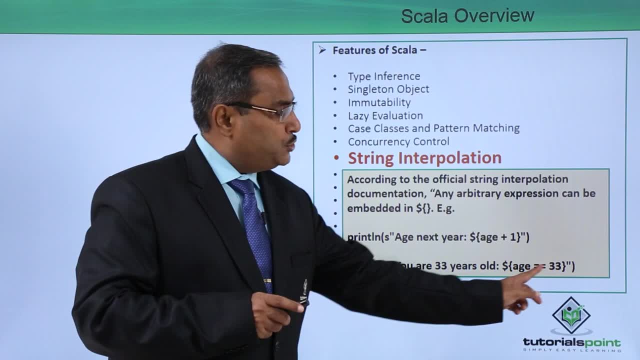 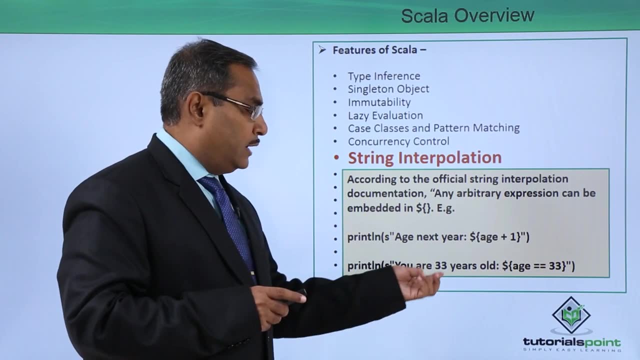 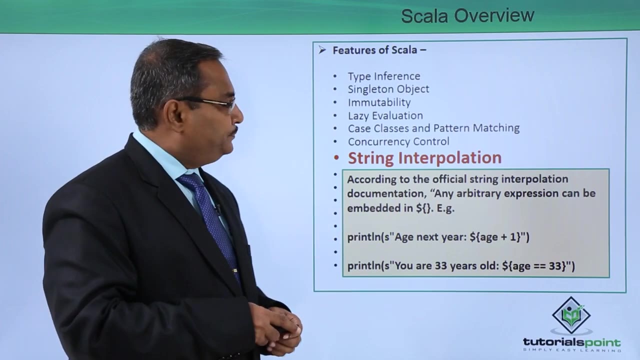 within the curly braces preceded by this dollar. so this expression will be evaluated. it will return either true or false and that will be treated as a string. and that then you, your. you are 33 years old. true or false will come when this code will get executed. so this is known as string interpolation. 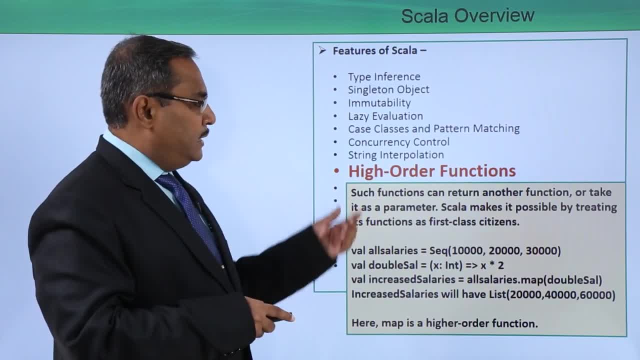 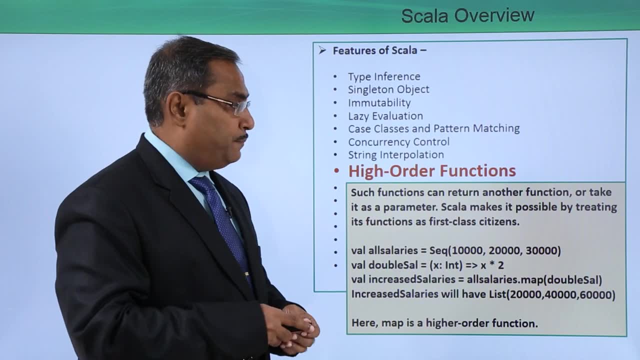 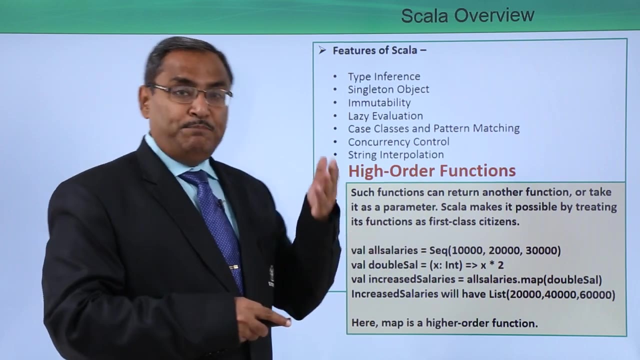 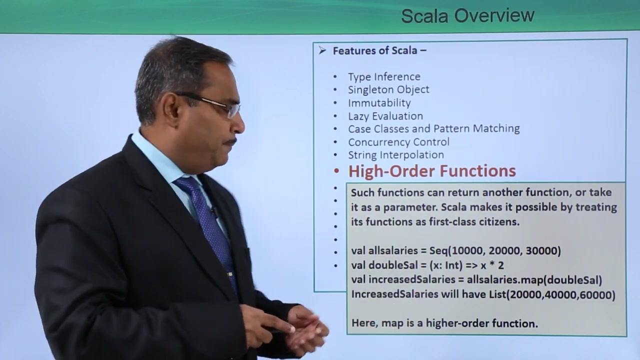 next, our next property is our high order functions. such functions can return another functions or take it as a parameter. so scholar makes it possible by treating its functions as the first class citizen. so in in this particular case, a function can take one function as input argument. a function can return a function as well. let us see one example here. so well, all salaries. 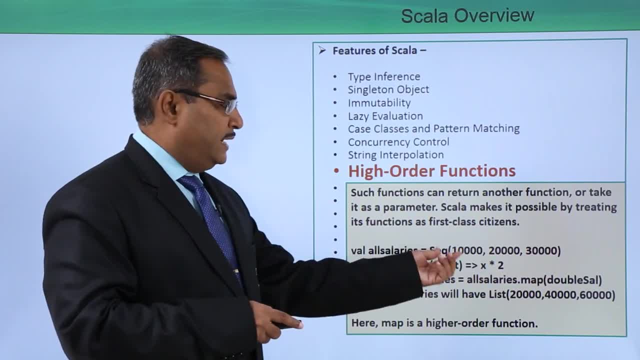 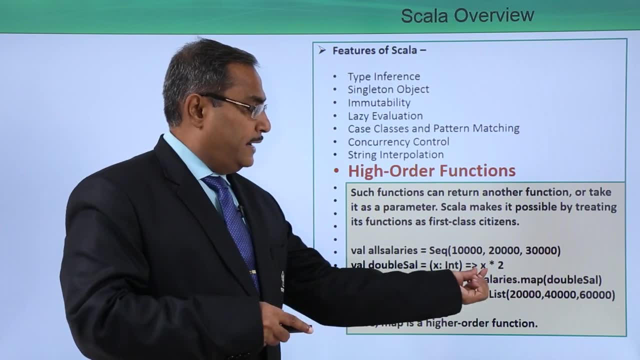 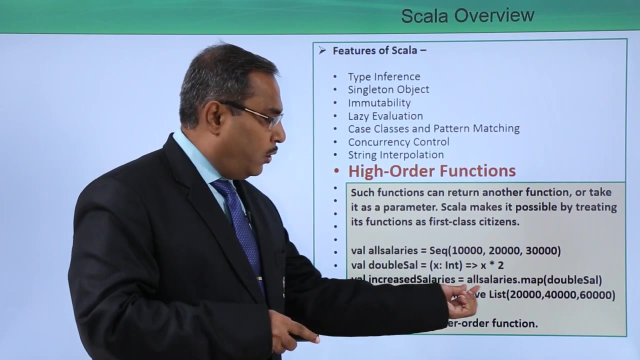 so here you have defined one sequence. so sequence is something like this: 10000, 20000 and 30000. so well, double cell is equal to x, which is of the type int, and here you see, it is just having the, the value x, star 2.. So well, increased salaries is equal to all salaries. dot map: What is? 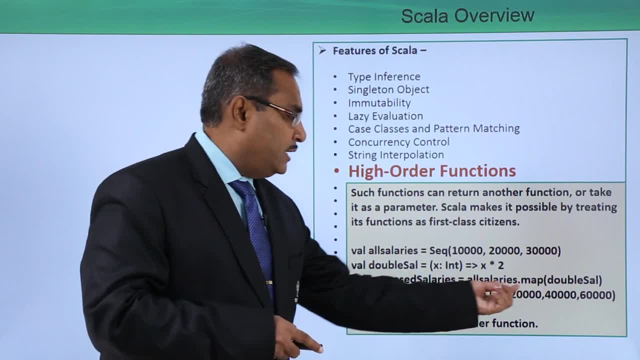 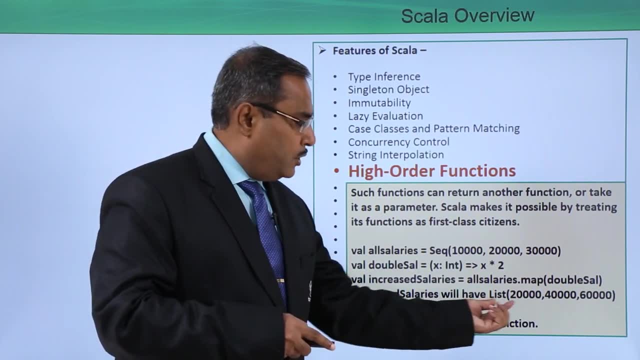 the all salaries, All salaries, is this particular sequence: All salaries dot map, double cell. So double cell is this one, So increased salaries will be, will produce one list in the output, that is 20,000,, 40,000,, 60,000, which are nothing but the double of this 10,000,. 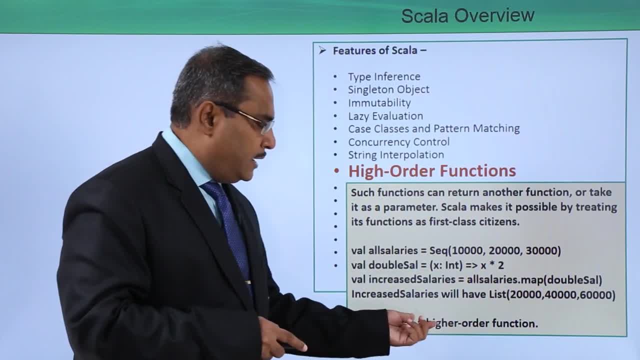 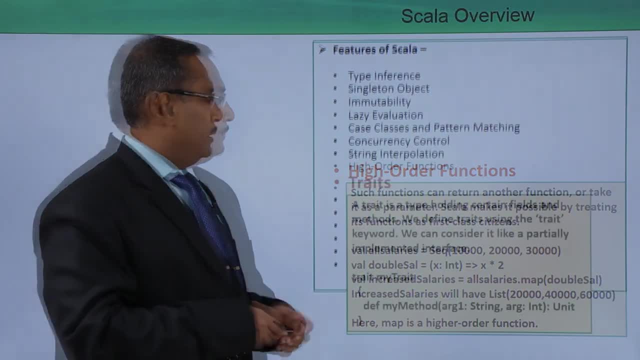 20,000 and 30,000 accordingly. Here this map is a high order functions we have used in this example, So the property is known as high order functions. Next property we are going to discuss is trait. A trait is a type holding certain fields and 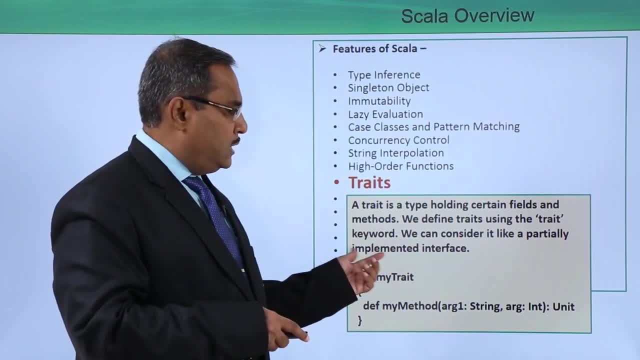 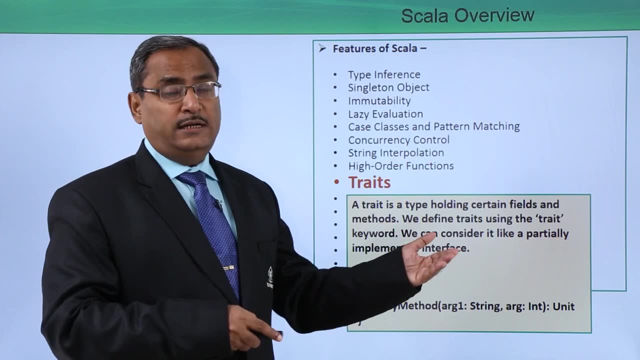 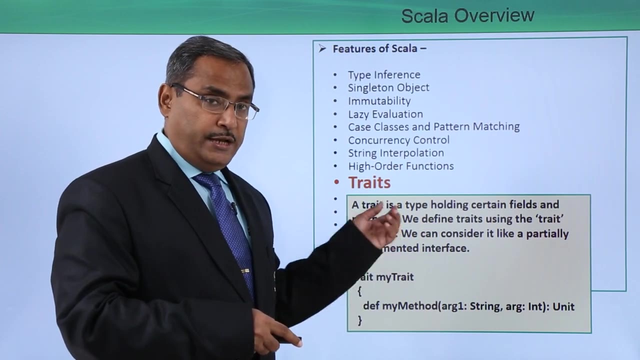 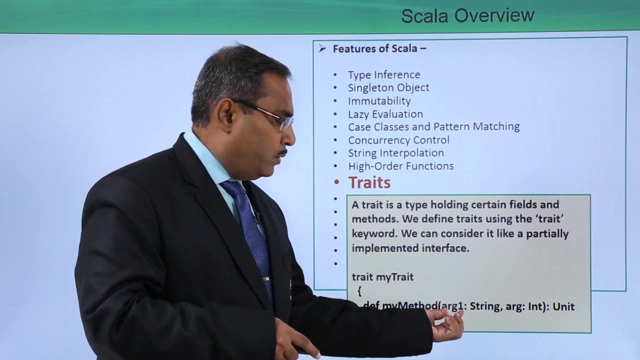 methods. We define traits using the trait keyword and we can consider it like a partially implemented interface. We had the concept of interface in our java, So here this particular partially implemented interface will be treated as a trait in our scalar programming. So trait, my trait. So here we are defining one method that is a my method argument one. 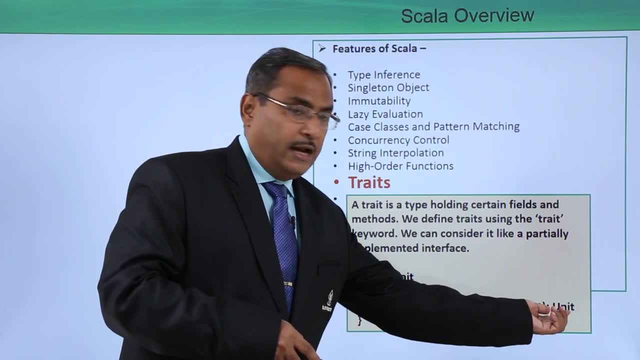 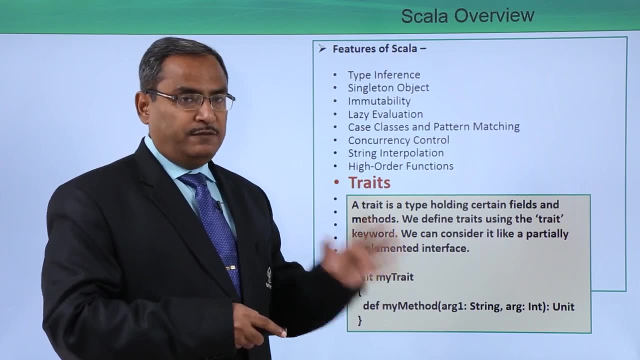 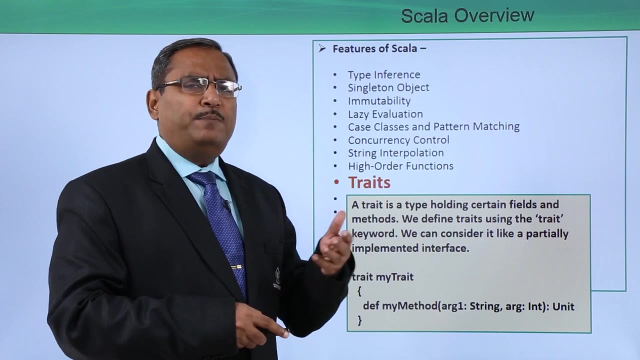 of the type string, argument will be of the type integer and which returns void or nothing. So in this way we are having this partially implemented interfaces which will be called as trait in our scalar programming, A class can. a class can implement multiple traits. 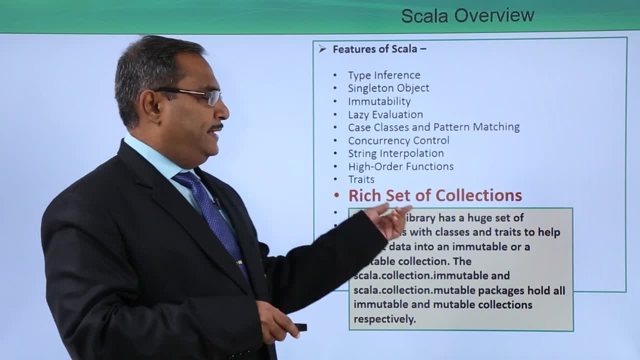 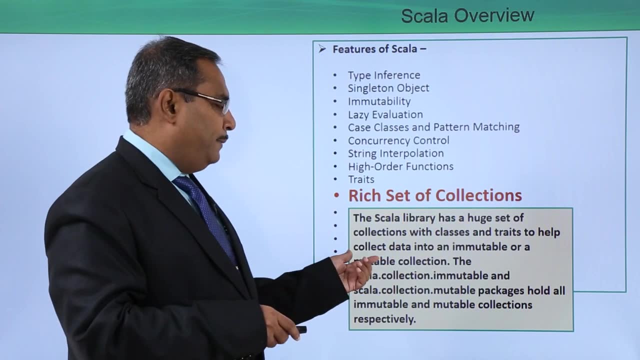 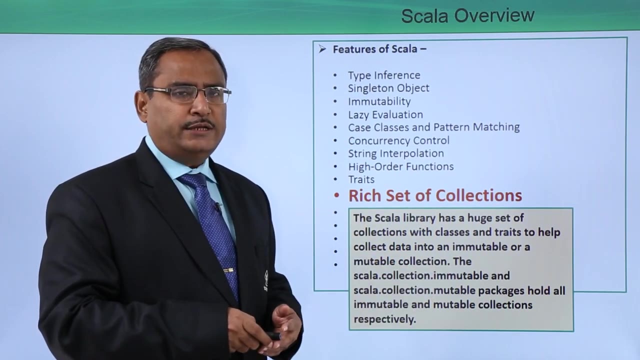 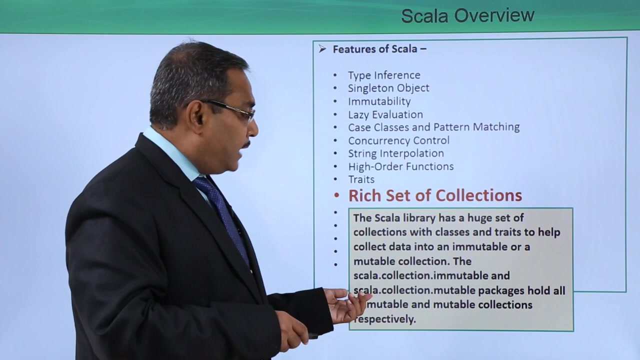 as when required. Next one is the reach set of collection. So this scalar library has a huge set of collections with classes and traits to help collect data into an immutable or immutable collections. So there are so many different collections are there in our scalar programming and the scalar dot collection dot- immutable and scalar. 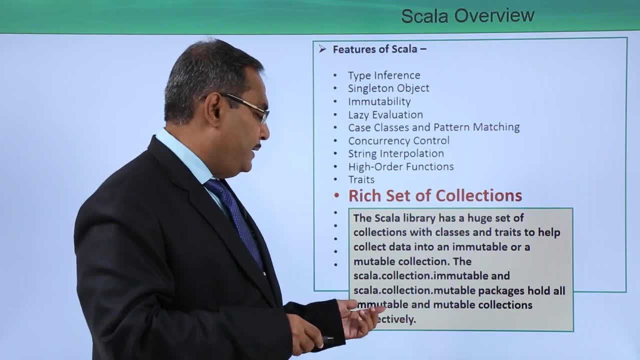 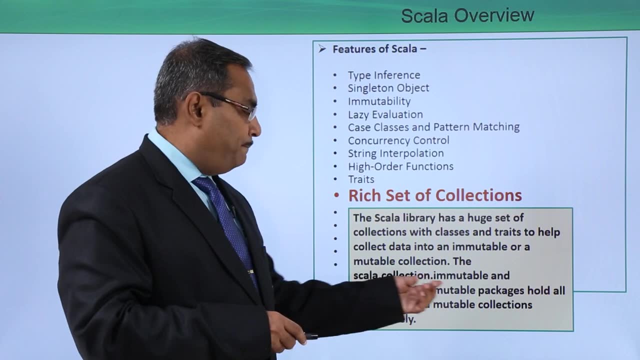 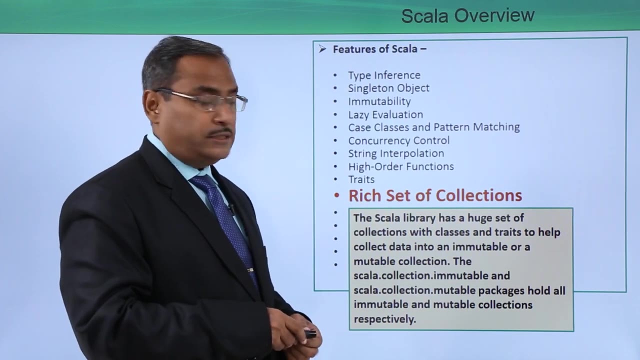 dot collection, dot immutable packages hold all the immutable and immutable collections respectively. So these are the two packages which are holding all the All the respective immutable and mutable collections which are being used in our scalar code. So reach set of collections. So the next property we are going to discuss is a functional programming. 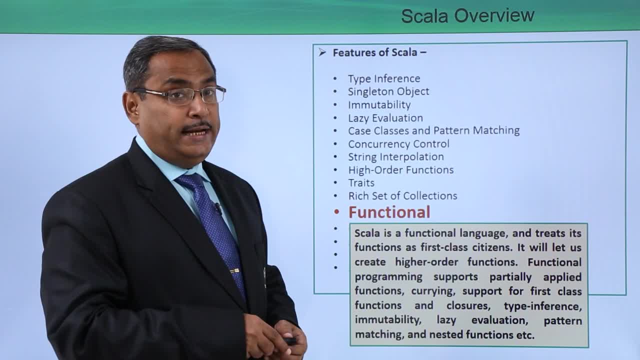 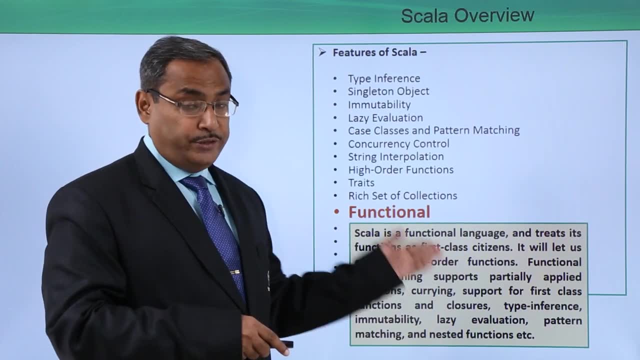 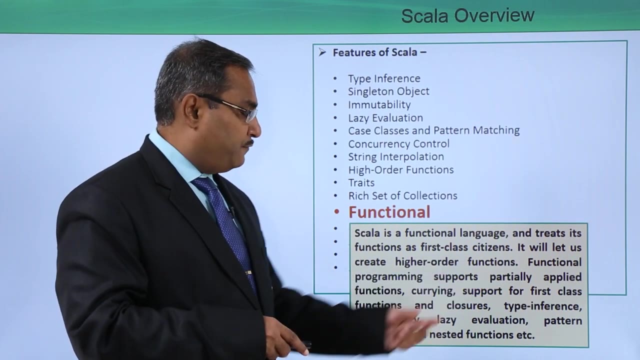 or functional language. So Scala is a functional language and it and treats it functions as first class citizens. It will let us create high order functions, which we discussed earlier. Functional programming supports partially applied functions, Adding support for first class functions and closures and type inference immutability. 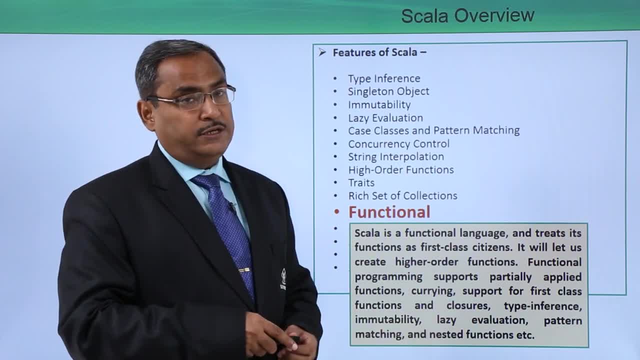 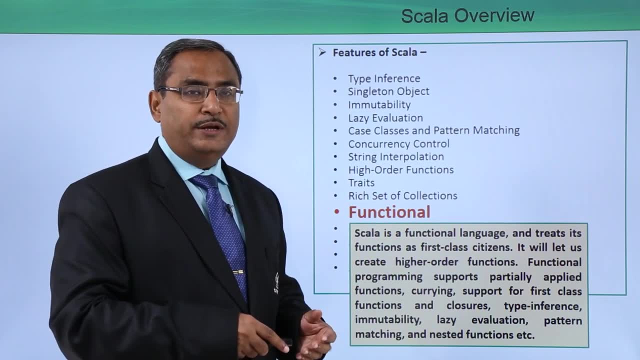 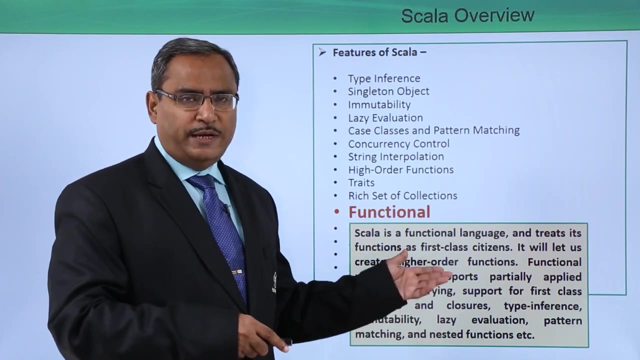 lazy evaluation, pattern matching and the nested functions, etcetera. So some of the features we have already discussed and other features will be discussing in our throughout this tutorial will be discussing this trait, this cutting these respective closures, the nested functions- all these things will be discussing, and now this is known as a functional programming. 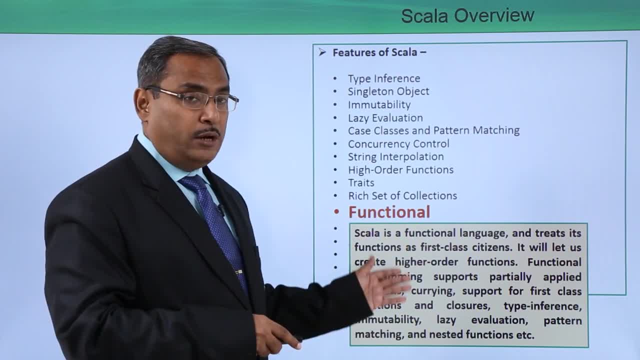 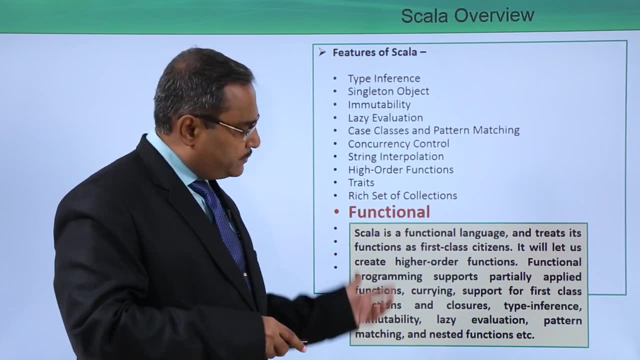 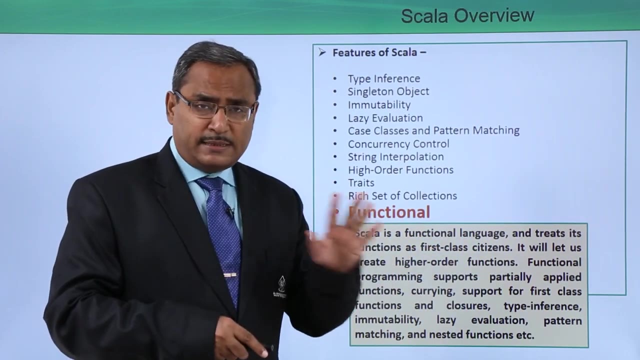 because functional programming Requires will have this particular properties and Scala supports all of them, and that is why it is called here. the main important statement. whatever has been written here is a functions as first class citizens, and this first class citizens were having a separate example, just. 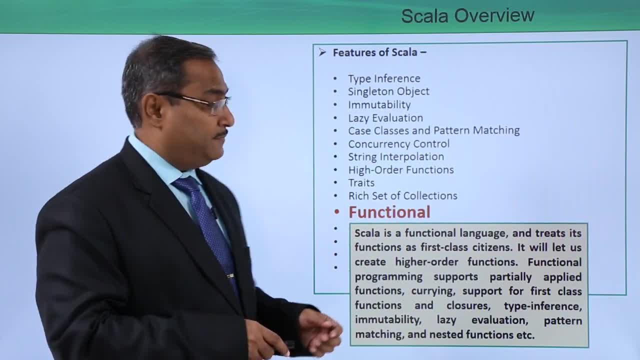 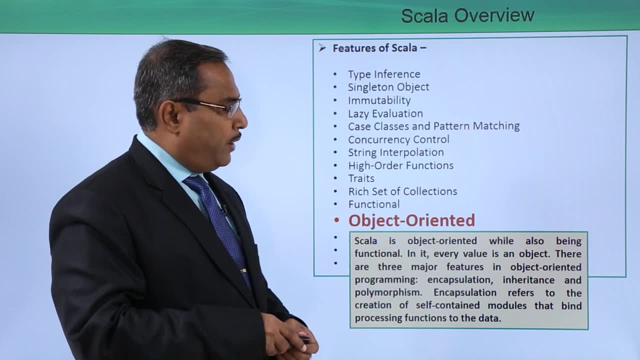 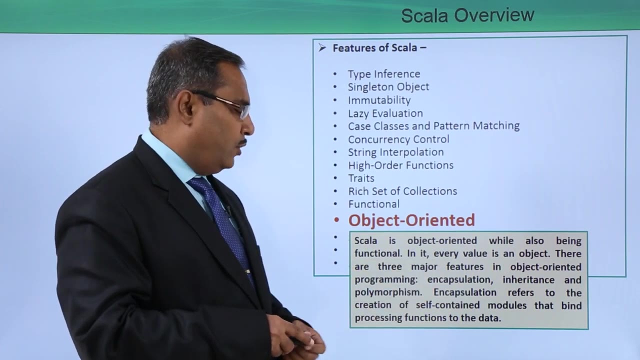 watch that one, we will be discussing why this functions are called as first class citizens. Next one is our object oriented. So Scala is object oriented while also being functional. In it, every value is an object. There are three major features in object oriented programming. 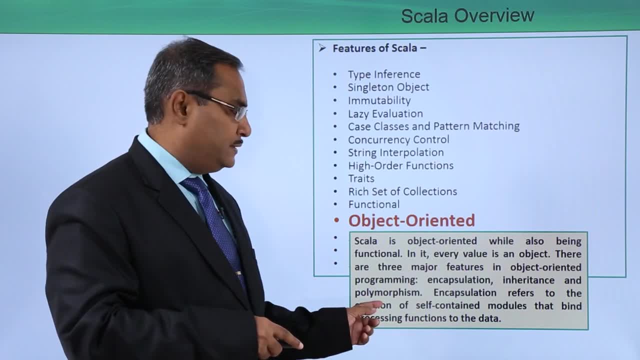 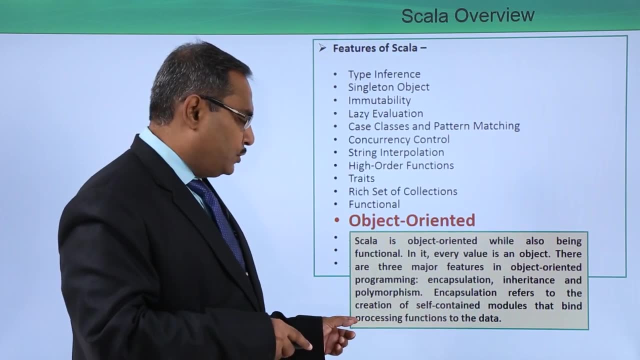 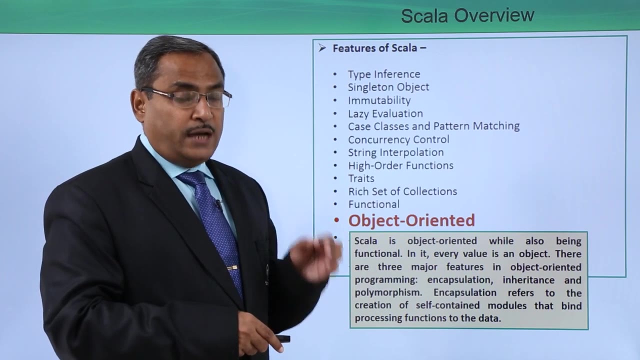 They are encapsulation, inheritance and polymorphism. Encapsulation refers to the creation of self content modules that bind processing functionals to the data. Next property is very important, that is, Scala is an object oriented language. So Scala is object oriented while also being functional. 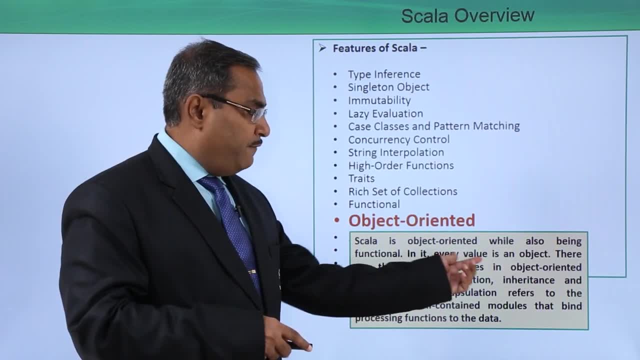 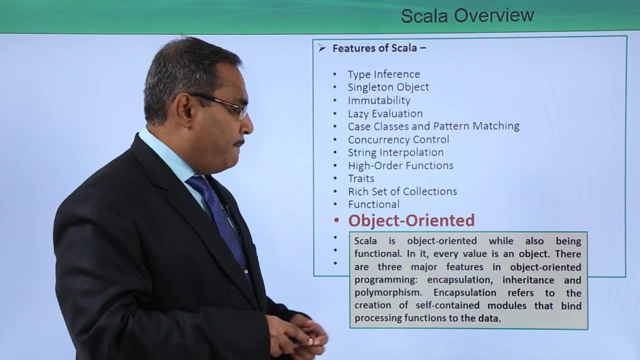 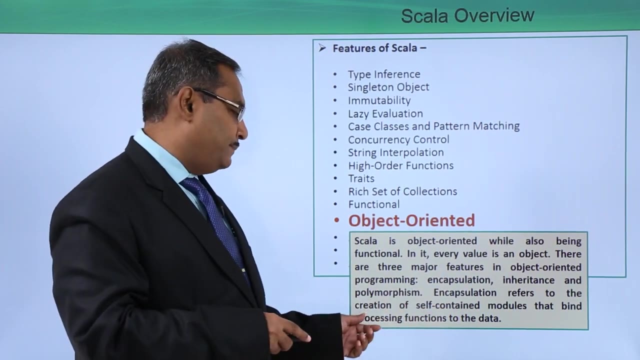 functional language and it is. every value is an object in Scala, So every, each and every value is nothing but an object. There are three major features in object oriented programming, and they are nothing but encapsulation, inheritance and polymorphism. And encapsulation refers to the 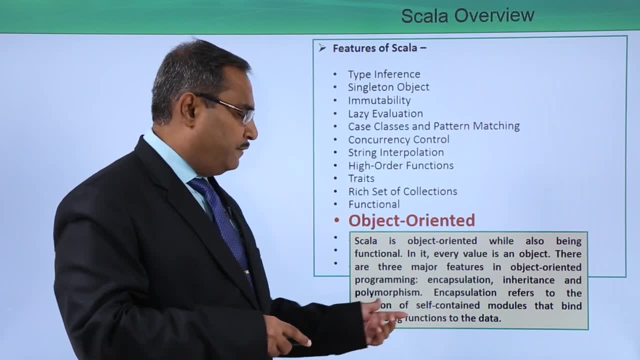 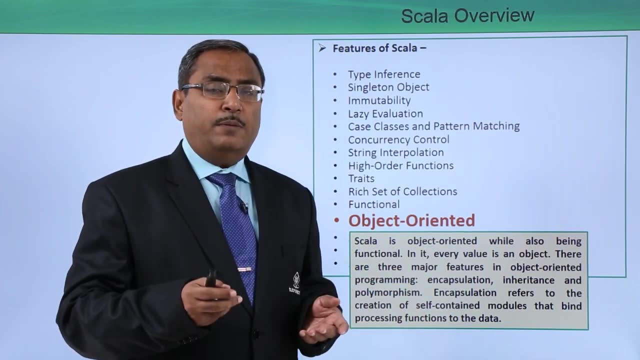 creation of self content modules that bind processing functions to the data. So here we are having the data, that is, the variables will be defining, which will be containing data, and set of methods which will decide what are the functions that you can carry out on the data, and that is. 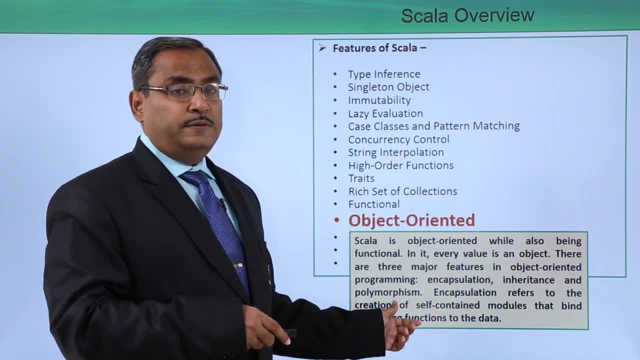 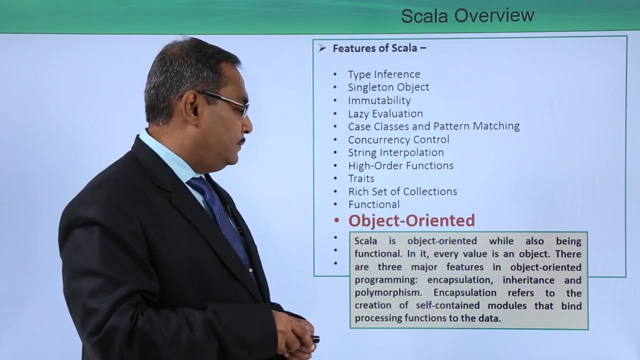 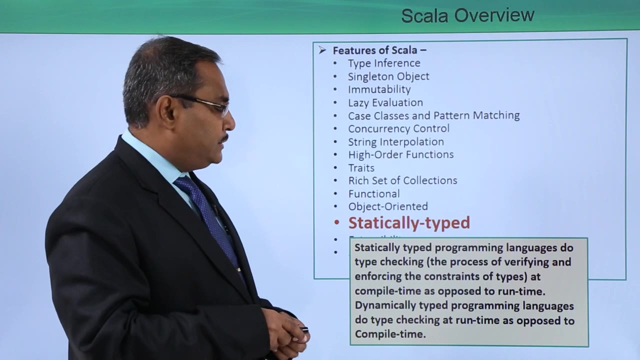 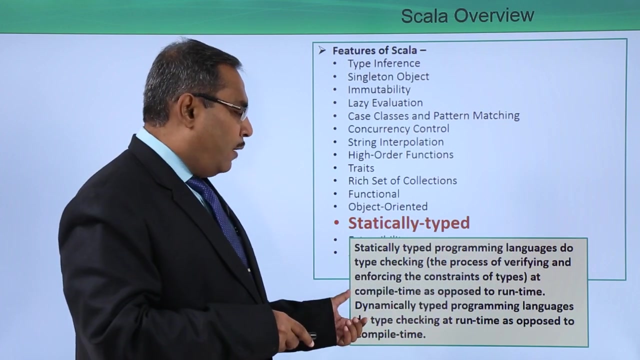 known as the encapsulation. So in case of Scala, one of the most important features is that it is object oriented programming language. Next one is the statically typed. So statically typed programming languages do type checking, the process of verifying and enforcing the constants of types at compile time as opposed to the run time. So all the 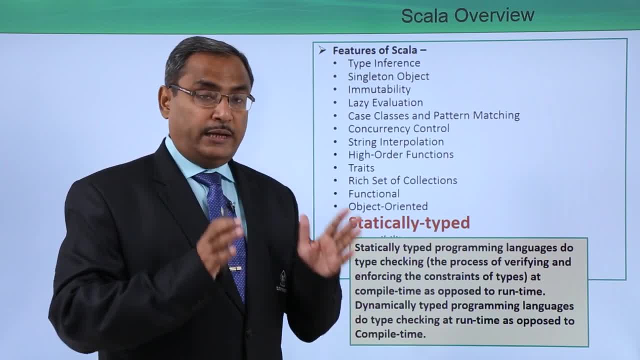 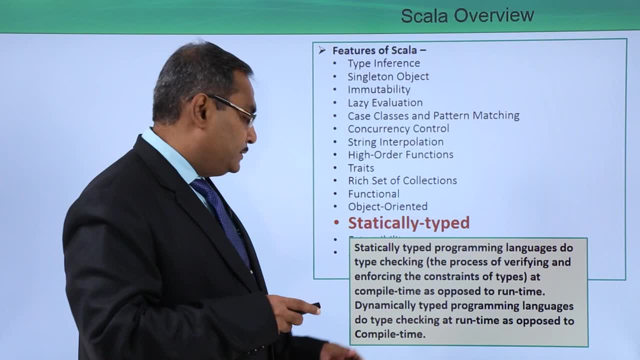 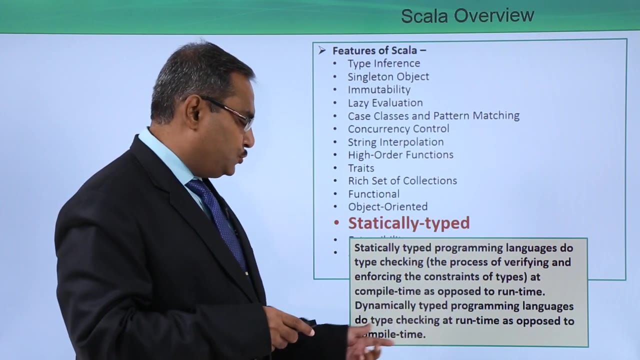 variable types will be defined during the compilation, during the compile time, not during the run time, and that is that is why these variables are known as statically typed variables. And dynamically typed programming languages do type checking at the run time as opposed to the compile time, and that will be known as the dynamically typed variables. But 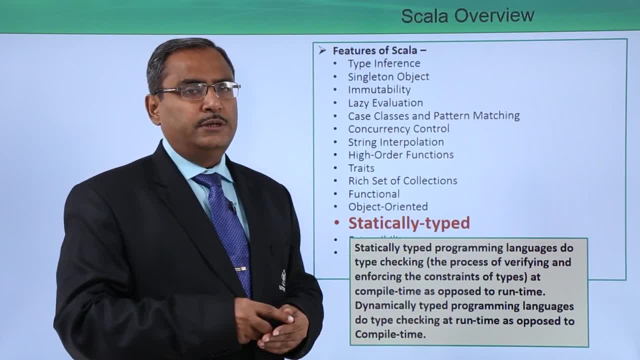 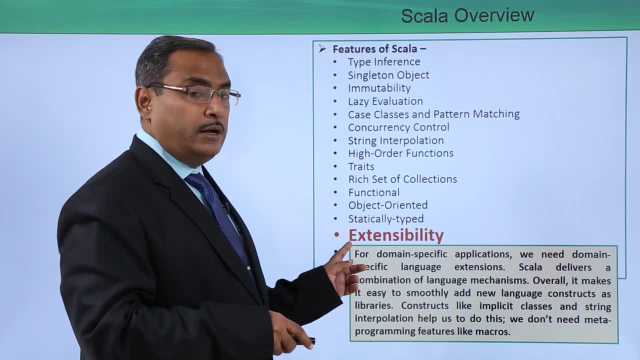 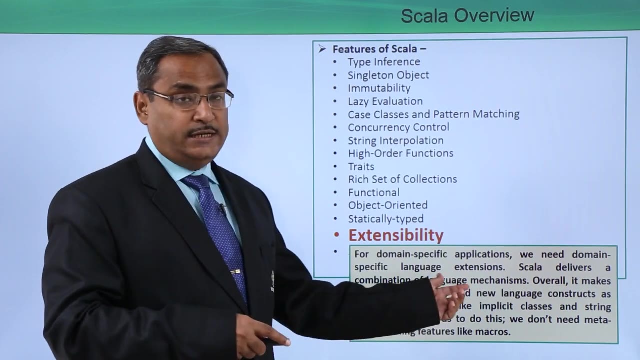 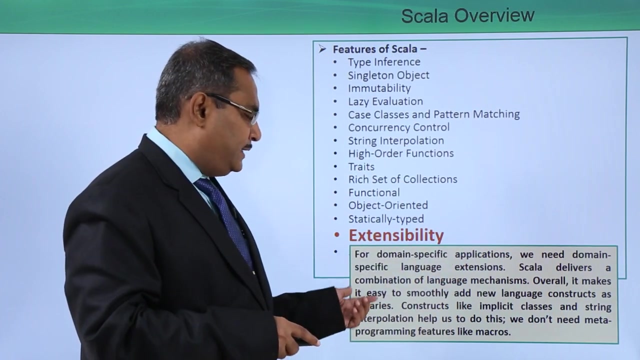 Scala supports statically typed variables. that means all the variables will have the data types defined during the compilation time We are having. next one is extensibility for domain specific applications. we need domain specific language extensions. Scala delivers a combination of language mechanisms. overall. it makes to it easy. 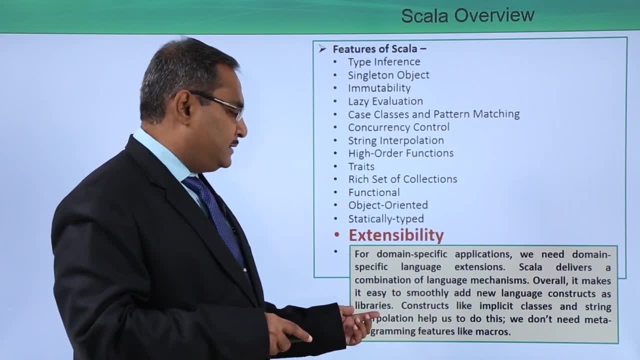 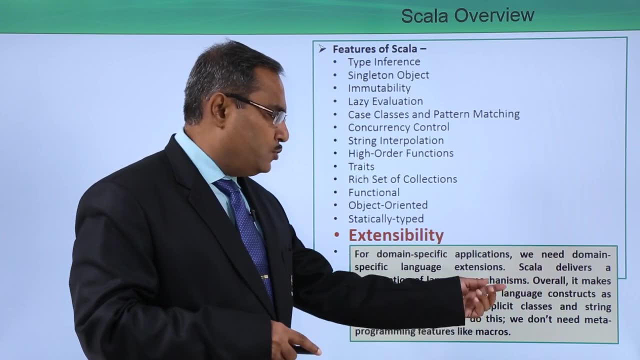 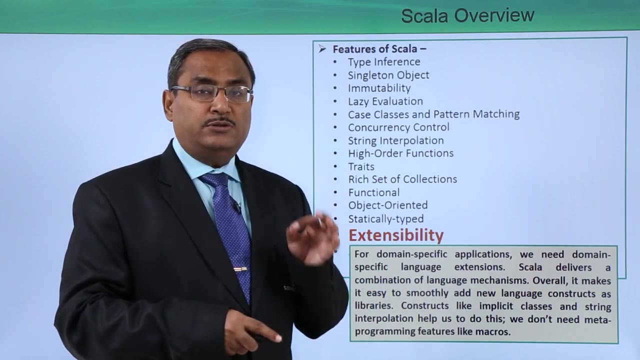 to smoothly add new language constructs as libraries and code. So we are having that way of constructs like the implicit classes and string interpolation help us to do this and we don't need meta programming like features like our macros. so if we, if we develop some applications with 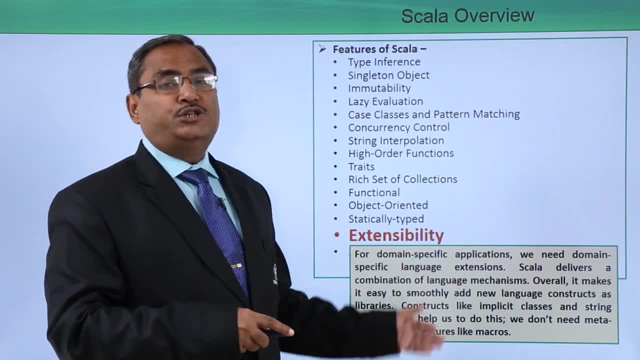 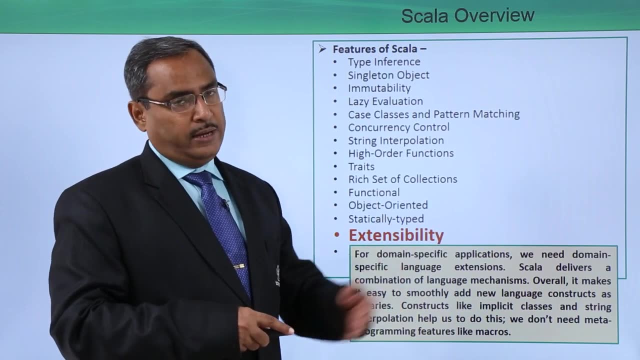 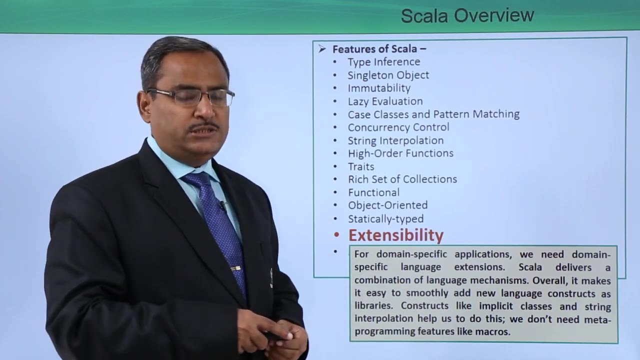 some special type of features. we can go for the extension extensibility features of scala can be used there and we can import certain different libraries in our scala and you can make the application on the according to the domain specific. so that's why the property is known as. 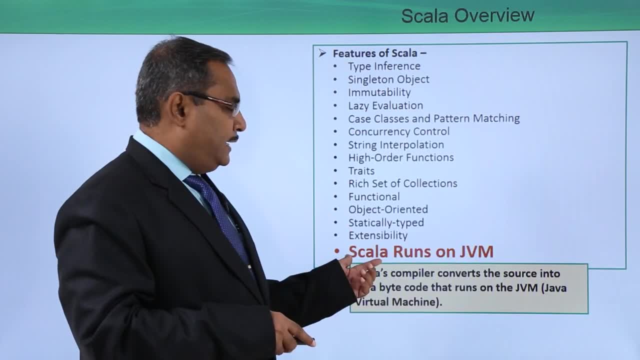 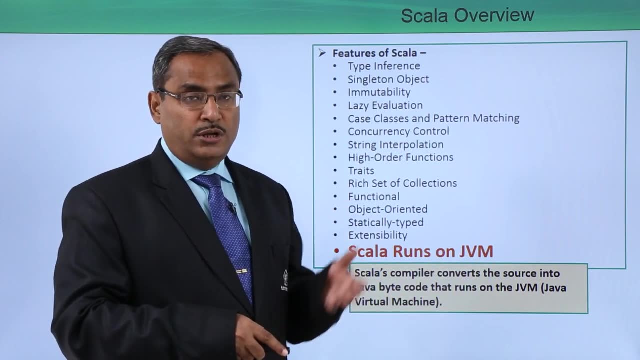 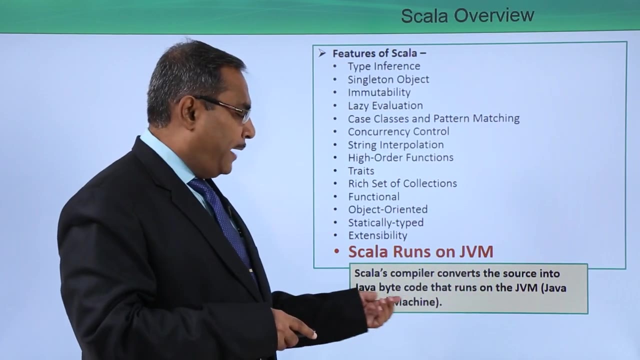 extensibility. the next property is the. that is the scala runs on jvm. the syntax of scala is very much alike to java and that's why it is getting more and more popularity. so scholars: compile, converts the source into java bytecode that runs on the jvm. that is a java virtual machine. 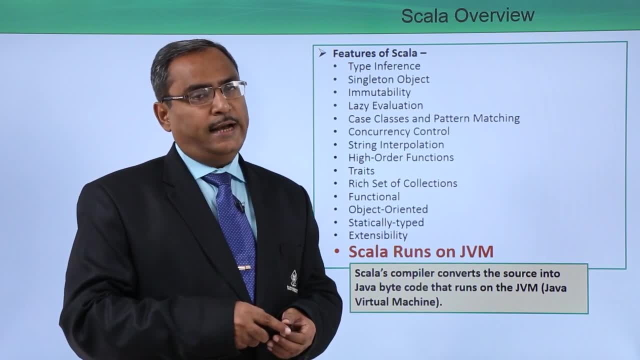 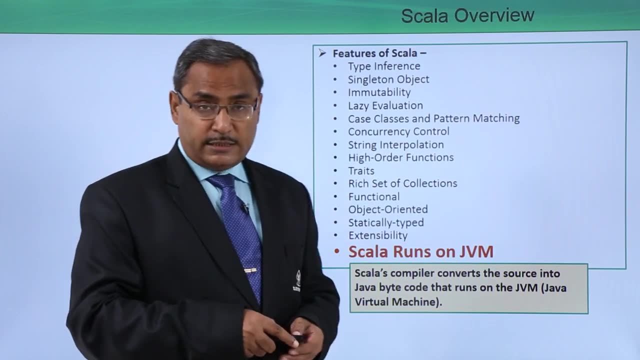 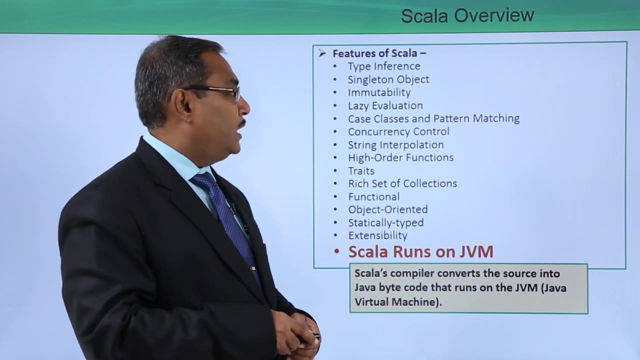 and you know that whenever we have having the bytecode format, and that is be making the language platform independent. so these are the features which you have discussed in this respective series of points. there is a 15 points we have discussed and they are the prime features of scala. so let us discuss two questions. 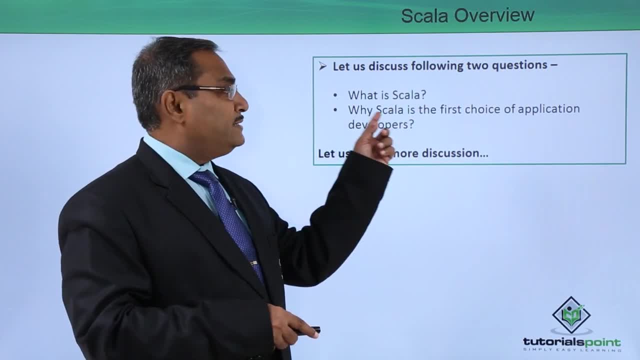 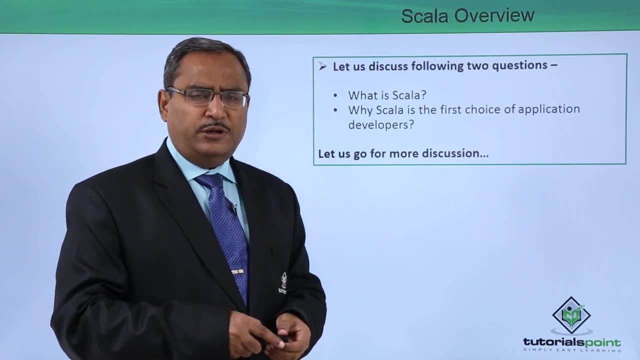 the first question is that: what is scala and why scala is the first choice of application developers. i think it is better let us go for some more discussion and in this particular section of this section of the video, we are going to talk about the first choice of application. 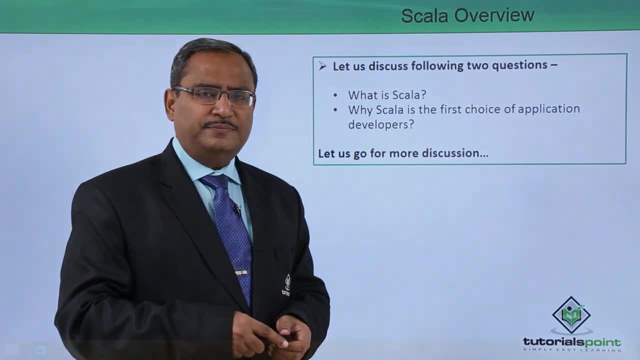 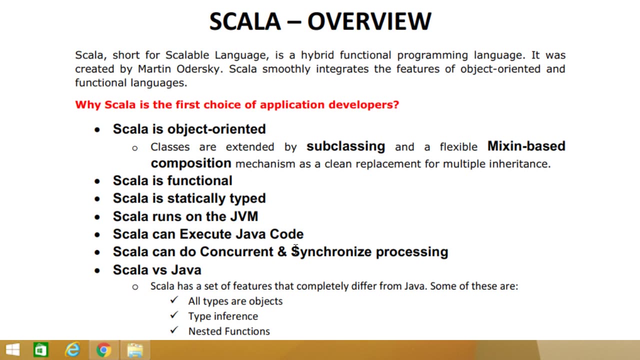 developers and in this particular section of the video, we are going to talk about the with some demonstration. So here is the discussion. Scala overview. Scala, short for scalable language, is a hybrid functional programming language and it was created by Mardin Odersky. Scala smoothly integrates the features of object-oriented and as well as 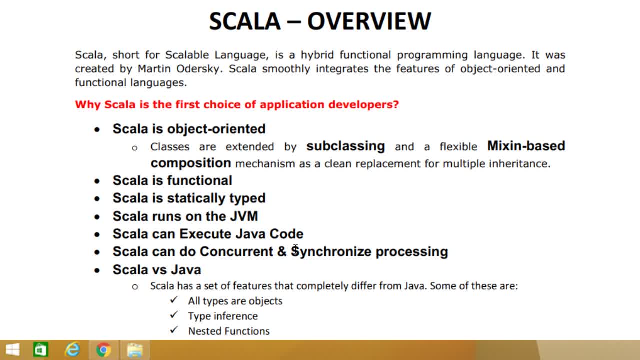 the functional languages. Scala is actually compiled to run on the Java virtual machine, that is, JVM. Many existing companies who depend on Java for business-critical applications are turning to Scala to boost their development, productivity, applications scalability and overall reliability. And we know that Scala is getting popular day by day. And why Scala is the? 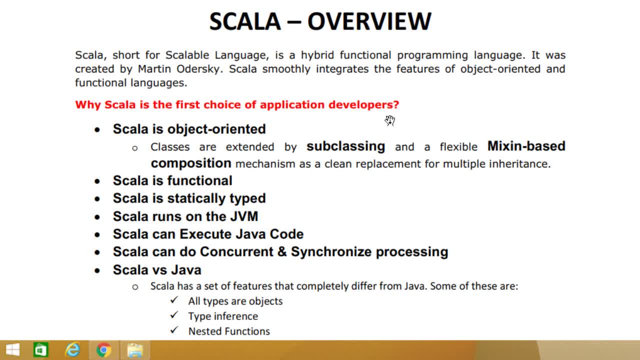 first choice of application developers. So that is the question, If we raise these questions. so here we are going to discuss some definite points. The first point is: Scala is fully object-oriented. So that means Scala is a pure object-oriented language, in the sense that every value is an object And types and 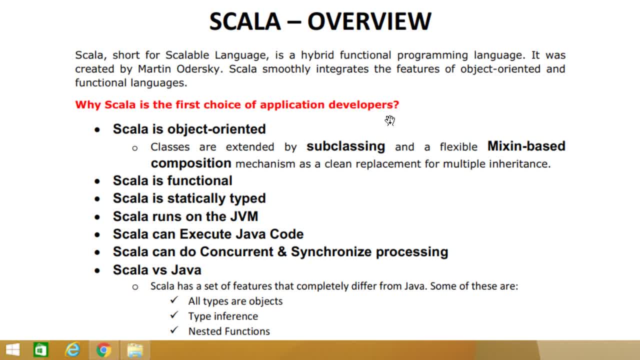 behavior of objects are described by classes and traits, and which will be discussed in our next videos detailing about this concept, And classes are extended by subclassing and a flexible mixing. The second point is: Scala is a function-based composition mechanism as a clean replacement for multiple inheritance. The next point we want to discuss is that Scala is functional. 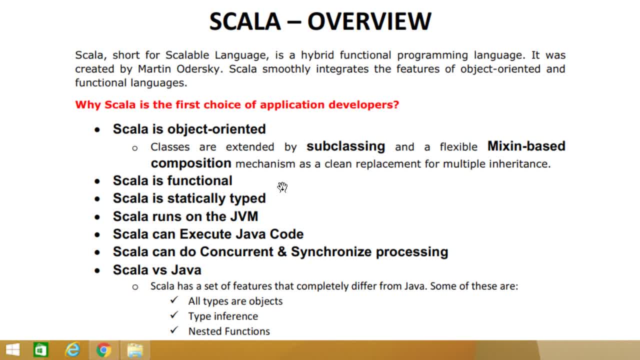 That is a very important point. So Scala is also a functional language, in the sense that every function is a value and every value is an object. So, ultimately, every function is an object. We are having a separate chapter on this function-based language, So let us 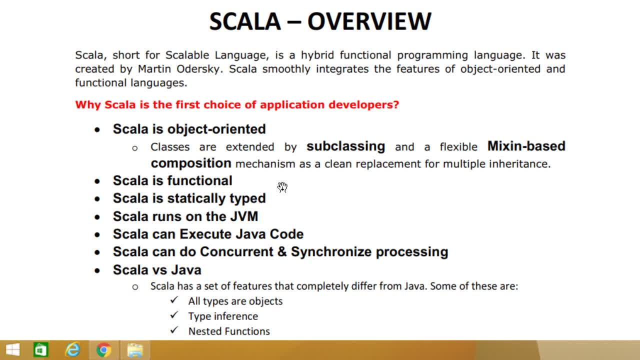 move on to the next point. Scala provides a lightweight syntax for defining anonymous functions. It supports higher-order functions, It allows functions to be nested and supports curring functions- And this concept we shall be discussing later also. So Scala is statically typed. So that is a very important one. That is, a Scala is statically. 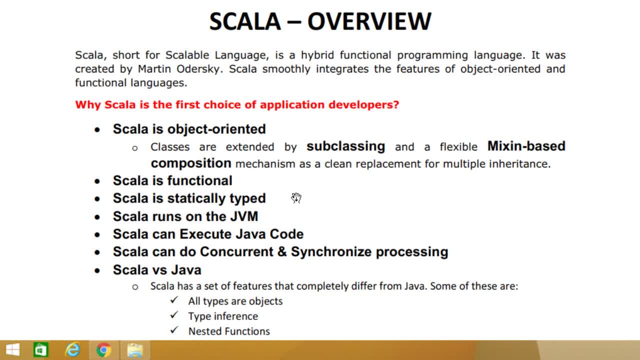 typed, So Scala, unlike some other statically typed languages. so here we are having, say, C, Pascal, Rust, etc. does not expect we to provide redundant type information. We don't have to specify a type in most cases and we certainly don't have to repeat it again. 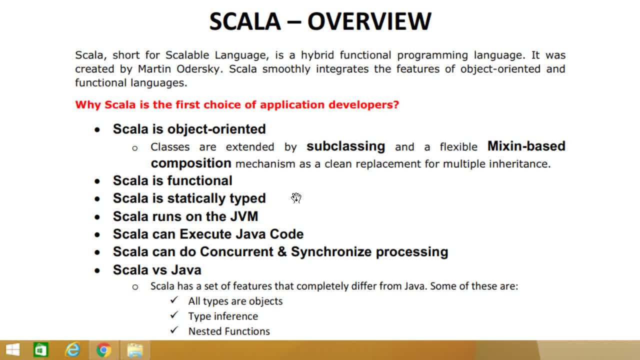 So in case of statically typed languages, the type of a variable will be determined during the compilation phase. So in case of statically typed languages, the type of a variable will be determined, not during the runtime of the application. Next one is: Java runs on the JVM, So Scala is compiled into Java bytecode which is executed. 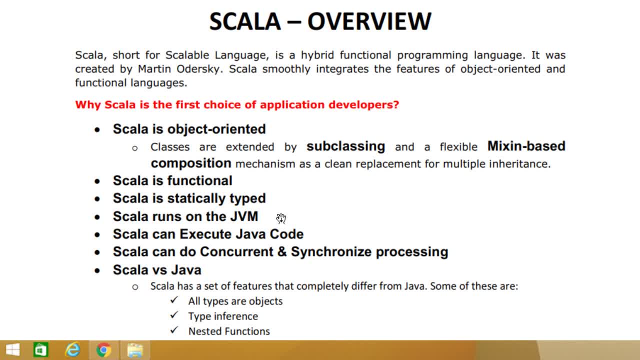 by the Java Virtual Machine, or JVM. This means that Scala and Java have a common runtime platform And we can easily move from Java to Scala. also, The Scala compiler compiles our Scala code into Java bytecode, So the Scala code is similar to Java's and then, which then get executed by the Scala command. The Scala. 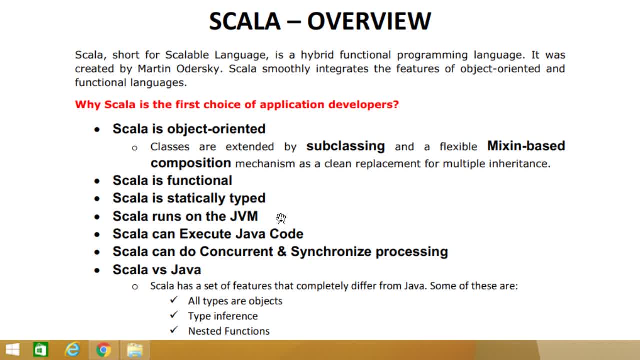 command is similar to the Java command. the java command because you know that in case of java program execution, at first we do the java c, we use the java c application for the java to convert that java code to the respective bytecode form and then for the execution of the java bytecode we usually issue the command java to. 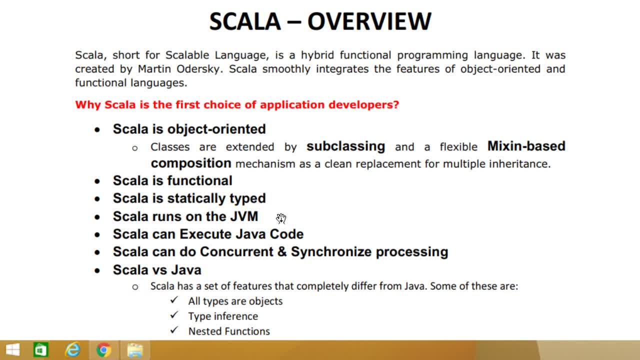 execute it. but in case of scala we'll be using the scala c, so that very application to convert this scala code to the bytecode format and later scala command will be used and that will execute our compiled scala code. so that is the main concept here. next one is that a scala can execute. 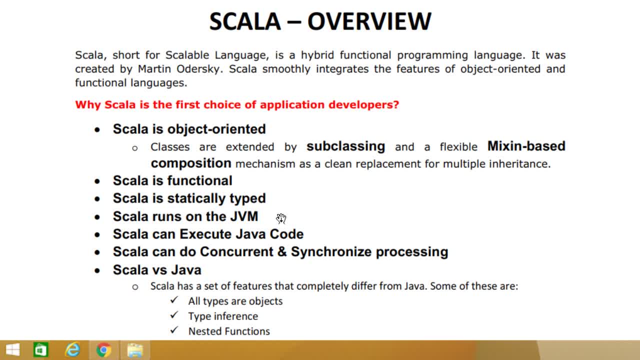 java code also. so scala enables us to use all the classes of the java sdk and also our own custom java classes or our favorite java open source projects. next point is scala can do concurrent and synchronize processing. so scala allows us to express general programming pattern in an effective way. it reduces the number of lines and helps. 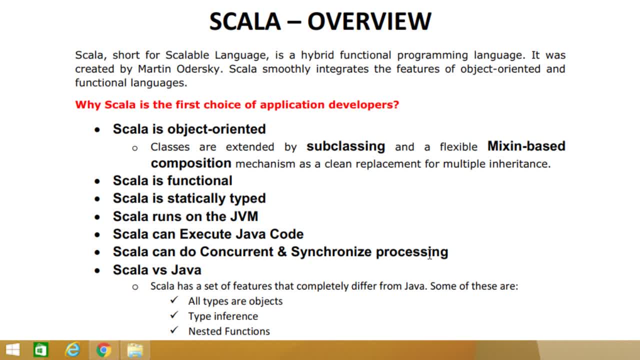 the programmer to code in a type, safe way. it allows us to write codes in an immutable manner and which makes it easy to apply concurrency and parallelism. that is a synchronization. there is a synchronization of the code. so that is the main concept here. next point is that a scala can do. 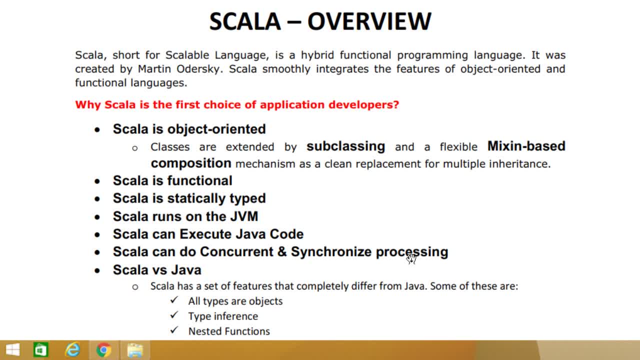 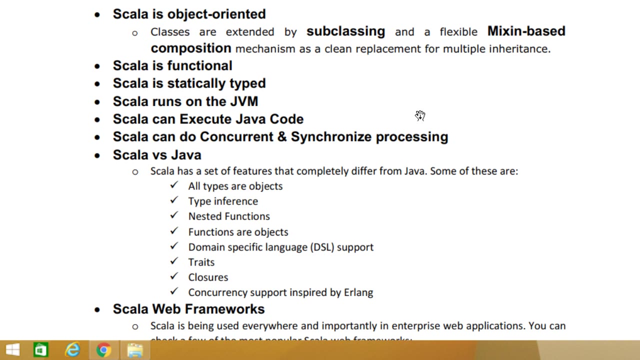 concurrent and synchronize. next one is: what is the difference between scala and the java? so scala versus java? so scala has a set of features that completely different from java, and some of these are all. types are objects, type inference, nested functions. functions are objects and domain: specific language, dsl, support threads, closers and concurrent. 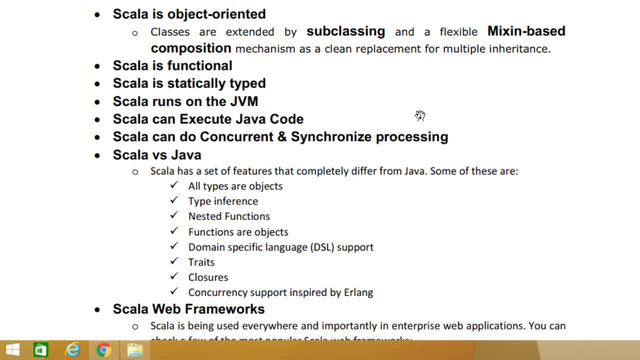 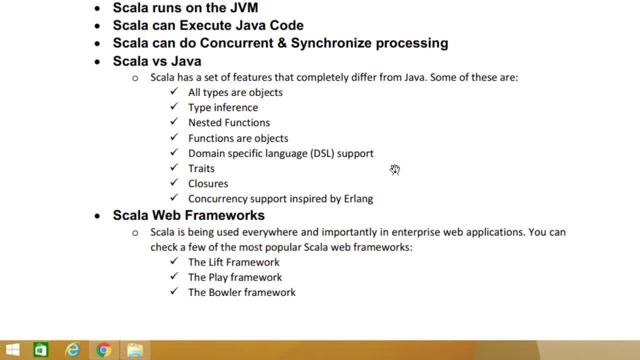 currency support inspired by erlang. so, regarding these aspects, we'll be having a separate video for that, for the detailed discussion. so the last feature is the scala web frameworks. scala is being used everywhere and, importantly, in enterprise web applications, and you can check a few of the 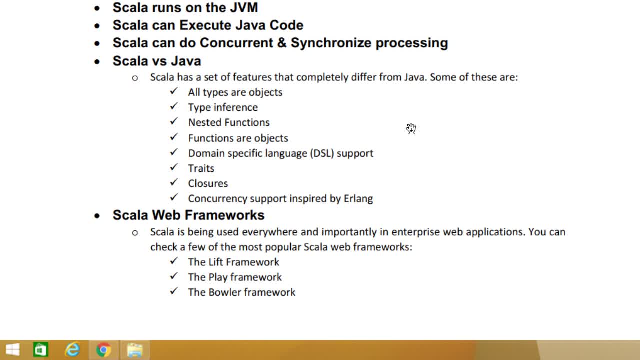 most popular scala web frameworks, and they are the, the libt framework, the play framework and the bowler framework. so these are the different features for which scala has become so popular nowadays. actually, frankly speaking, if you were earnestly looking for a technique to simplify your code for object oriented programming projects, but want to stick to functional programming, scala is. 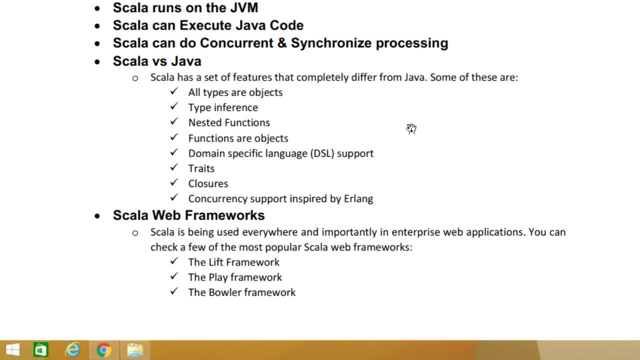 one of the most excellent choices you can opt for, and, whether you work with c and c plus plus java, scala based big data programming is one of the most excellent choices you can opt for, and, whether you work with c and c plus plus java, scala based big data programming is one of the most excellent choices. 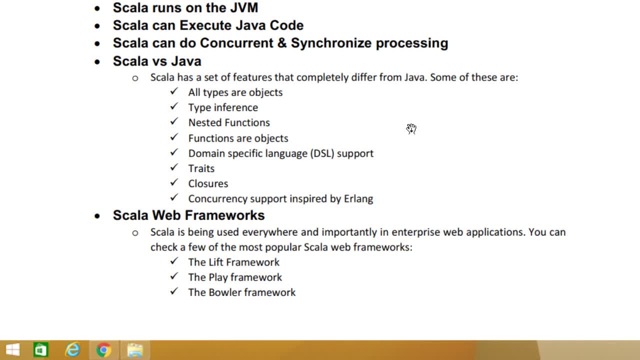 widely reversed for its high speed and expressiveness, with a cleaner and simpler design and syntax. scala runs successfully on jvm and brings you the efficient ways of handling the hues datasets. and brings you the efficient ways of handling the hues data sets and that's why in different big data related applications. 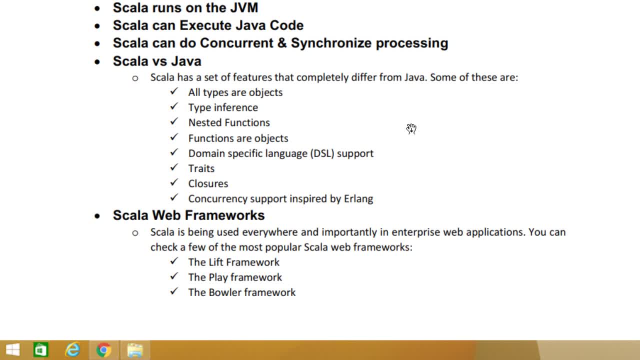 scholars. color programming language is getting used widely and it offers a smoother historical data security. hinaus in data security for applications or transitionNodeц and swantheral platform that finds the expert. samma web application, the website of game idea. integration of object-oriented and functional languages- whatever you have discussed right now.